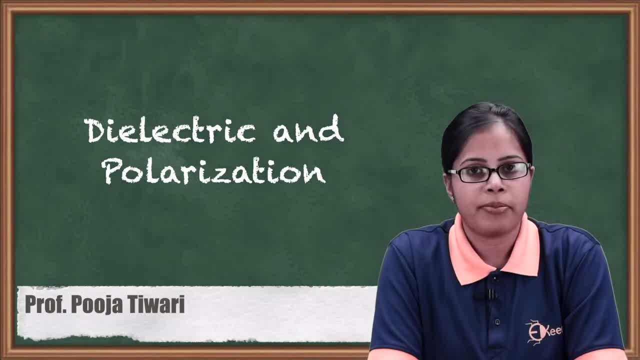 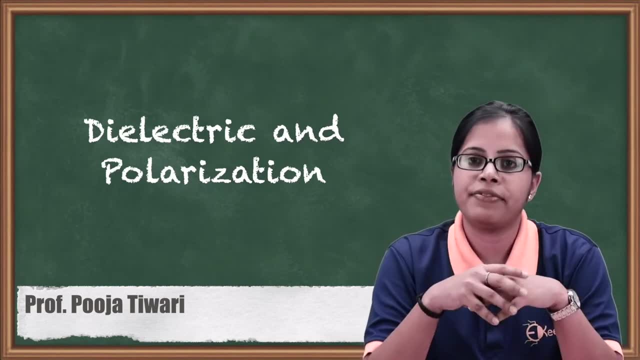 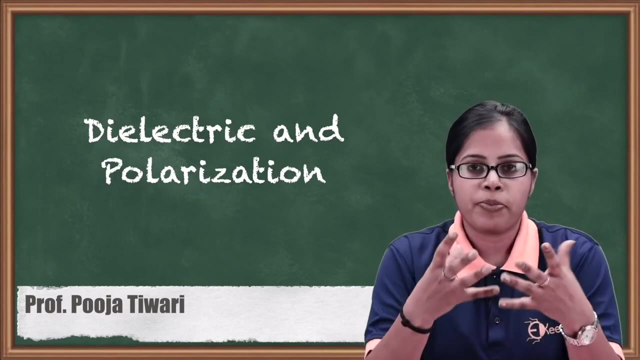 Hello friends. so today we are going to specifically talk about. what do you mean by dielectric materials? Are they very much different from whatever we have discussed in the previous sections or school sections? Secondly, we are going to talk about the process called as polarization, which occur in dielectrics. 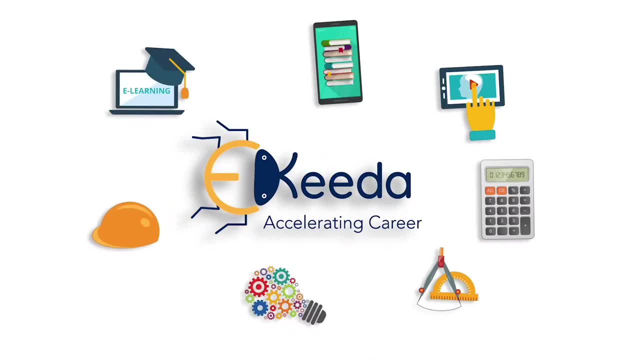 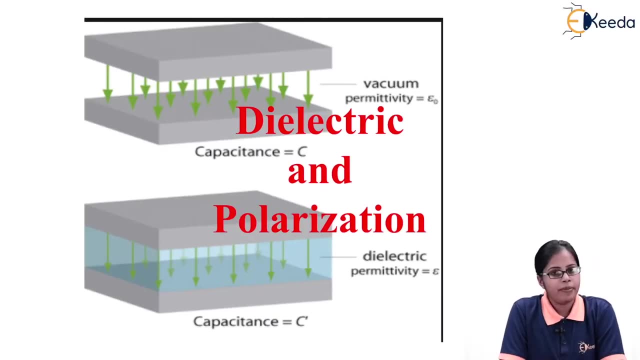 So, starting with the concept of dielectric and polarization, the concept comes. is what do you mean by dielectric? Like the basics comes from, like we say materials are going to have two classifications: One is conductor and the other one is insulator. But when we talk about insulators, 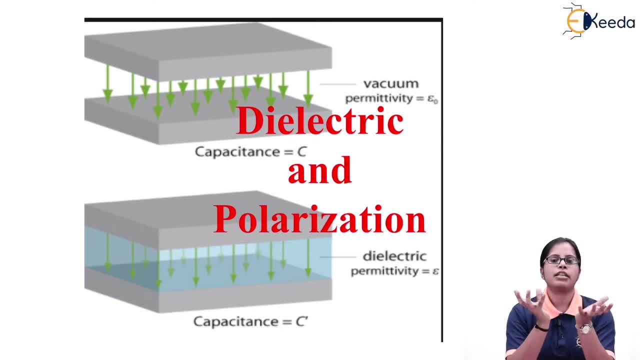 or conductors. we are going to talk about the concept of dielectric and polarization. These are two classifications of the material which are dependent on availability of free charges, Like if we say: I have a material in which there is a presence of free charge. 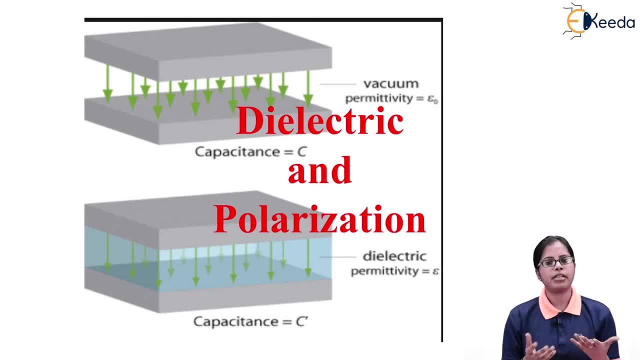 that material is considered to be conductor. But if I have a material in which the material does not consist of free charges, or you can say does not consist of free electrons, those type of materials are considered to be insulators, Or you can say the non-conducting material. So the materials having non-conducting nature, 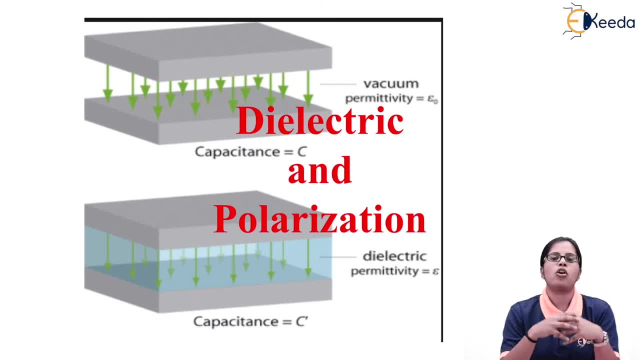 or insulating nature are also called as dielectrics. So when you talk about dielectric, dielectric are nothing but the non-conducting material, or you can say the insulating material which has no availability of free charges or free electrons. So when we talk about insulating, 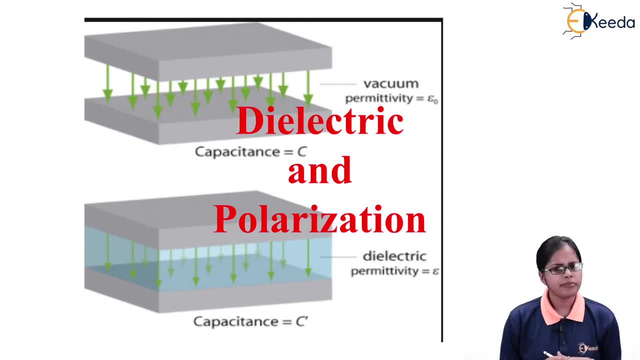 material or we talk about dielectric. we are going to talk about the non-conducting material. We simply say that there is no free charges, no free electrons in that. So we can consider that non-conducting material to be a dielectric material. But when we are talking about dielectric, 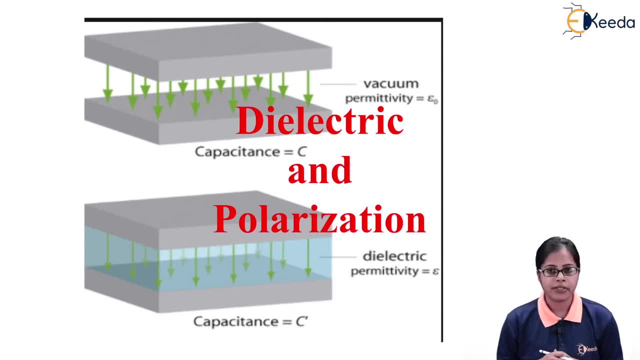 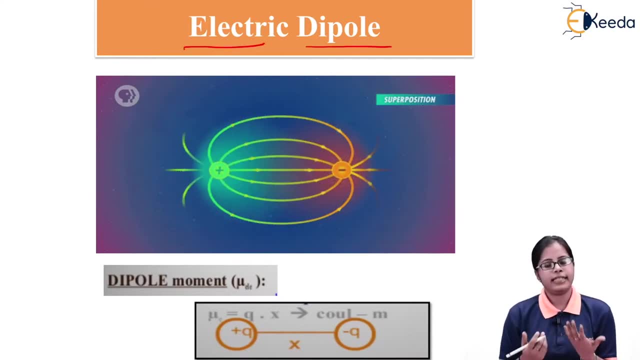 material, we need to talk about an important parameter, which is called as electric dipole. Now, when we talk about electric dipole, let us see what do you mean by electric dipole Before starting with the concept, as we are aware that there are two types of electric charges available in nature. One is 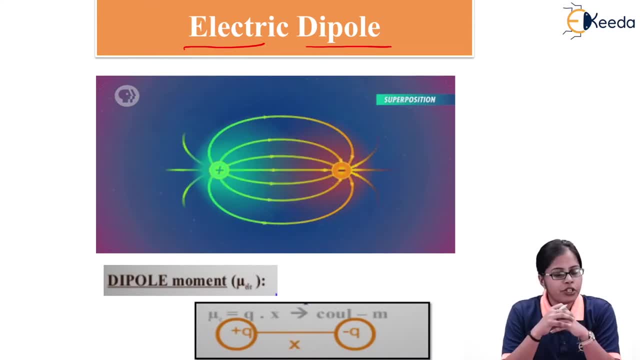 positive electric charge and the second one is negative electric charge. So whenever we talk about the types of electric charges, there are two types of electric charges: positive electric charge and the negative electric charges. Secondly, when we talk about like electric charges, 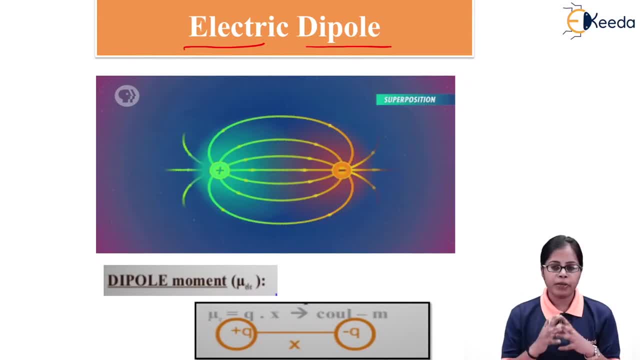 they have proper repulsion between them. and if I have, unlike electric charges together, it is going to have force of attraction between them. But if I want to form an electric dipole now, to form an electric dipole I must make use of two charges. Like I can make use of a charge plus q situated at a. 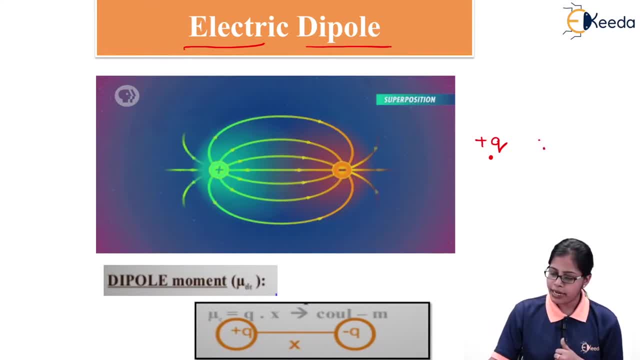 particular point and I can have a minus q charge, and I can have a minus q charge and I can have a minus q charge situated at another point b. So I have two points, a and b, plus q charge situated at point a, minus q charge situated at point b. As you can see, I have not drawn. 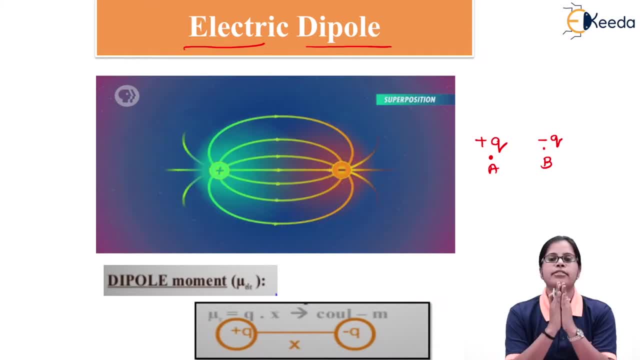 the two charges coinciding with each other. The two charges are separated by a certain distance. So when we talk about the two charges, that is, plus q and minus q, as we can see, the charges are opposite, That is, one charge possesses positive charge and the second charge 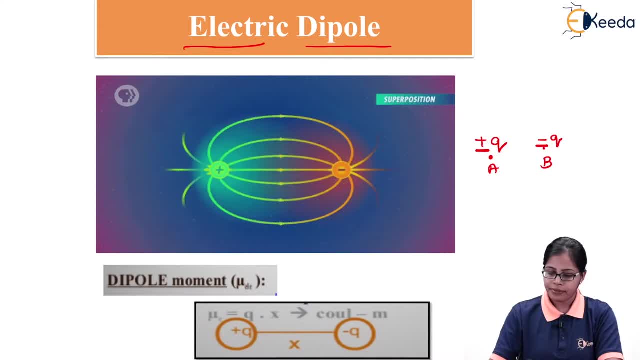 possesses negative charge, But if we look at magnitude of the charge, it is taken to be the same. So I have considered two charges of equal magnitude, that is q, but the signs are opposite: One is a positive charge and the other one is a negative charge. So if I have two equal and 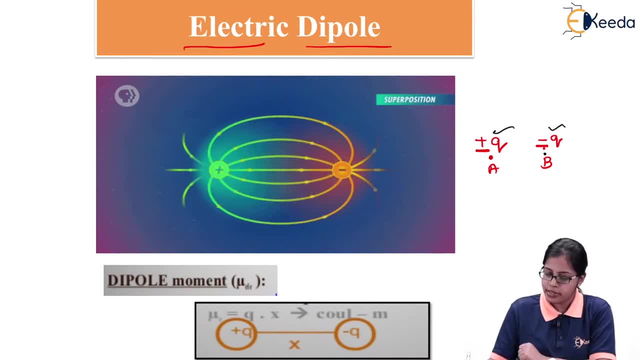 opposite charges which are separated by a certain distance. it leads to the formation of electric dipole. So, as you can see in this diagram, I have considered a positive charge over here and a negative charge over here, and these two charges have equal magnitude. 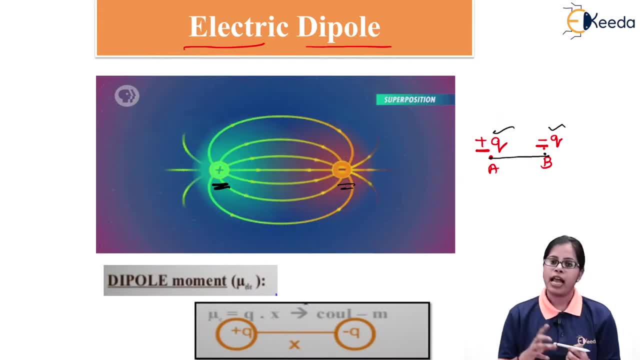 but they are of opposite charges, That is, one is positive charge and the other one is negative charge and they both are separated by a finite distance and if all the conditions are getting satisfied, that is, if the two charges are of equal magnitude and opposite. 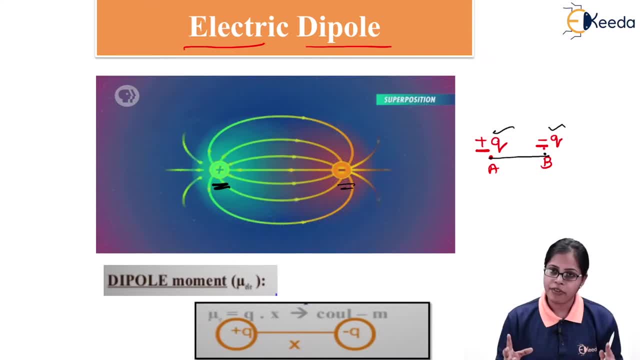 charges. secondly, if they are separated by a certain finite distance, then it leads to the formation of electric dipole. So if these two conditions are getting satisfied, we say that there is a formation of electric dipole. So if you look at electric dipole you can. 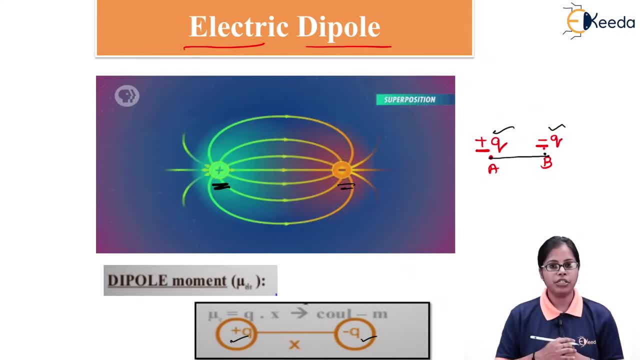 see in the diagram, I have a plus q charge and a minus q charge. They both are of equal magnitude, separated by a finite distance of x, and whenever we take the product of magnitude of one of the charges and the distance between them, as you can see in the diagram, the magnitude 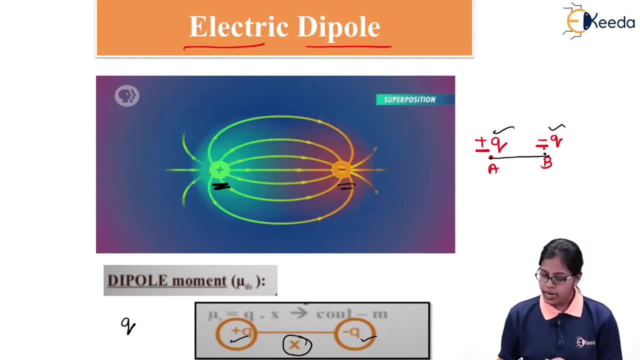 of one of the charges is considered to be q, The distance between the two charges is taken to be x. So if I take the product of q and x, I am going to get a quantity which to be written as dipole moment. so if we want to talk about dipole moment, dipole moment is nothing. 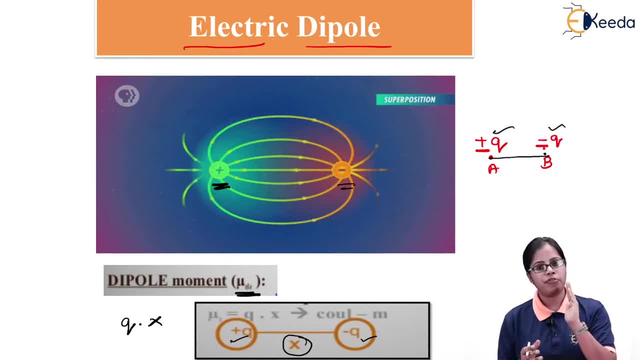 but mathematically taken as product of magnitude of one of the charges and the distance between them. as you can see in the diagram, the magnitude of one of the charges taken to be q and the separation between the two charges is x. so the product of the two is going to give me a term. 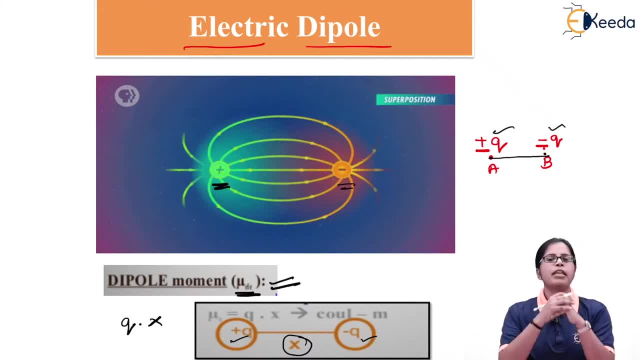 called as dipole moment. so this is a mathematical way of writing the dipole moment. but if it is asked, what do you mean by dipole moment? physically, it means that the strength of electric dipole- if i want to talk about the strength of electric dipole, that value of the strength of electric 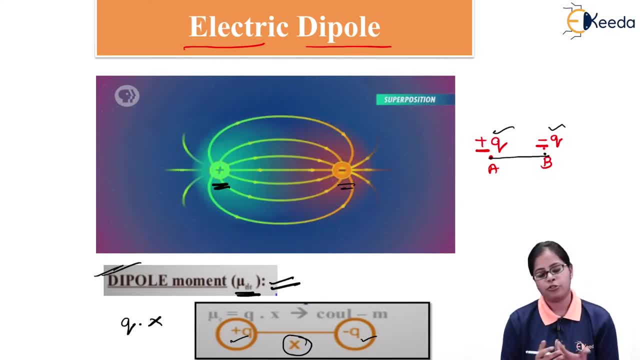 dipole will be given in terms of dipole moment. so mathematically, dipole moment is given by the formula mu is equal to magnitude of one of the charges, times the distance between the two charges mathematically. secondly, if i want to understand, what do you mean by dipole moment? it is the 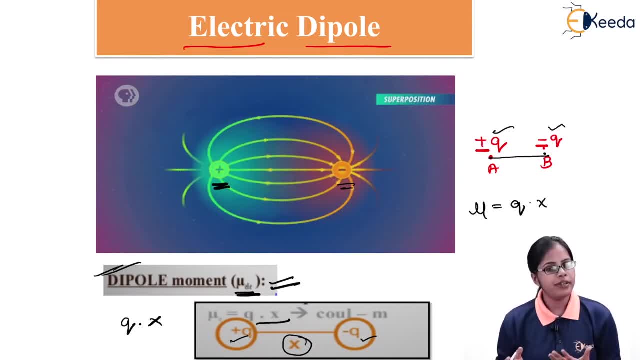 strength of the electric dipole, which i have conceded. that is what we talk about, the dipole moment. now, if you look at the unit of dipole moment, that is of mu, in that case the unit is going to be obviously dependent on the formula: the charge has a unit of coulomb and x has a unit of meter. so the coulomb meter is going to be the unit of. 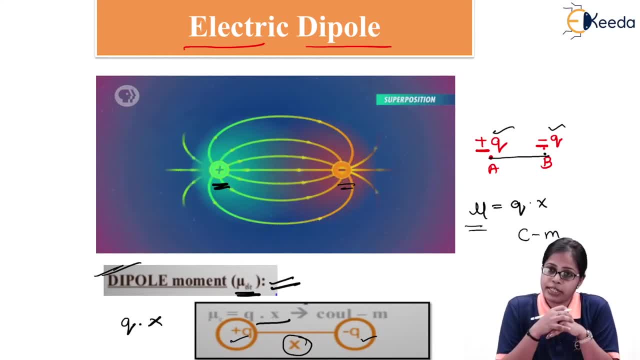 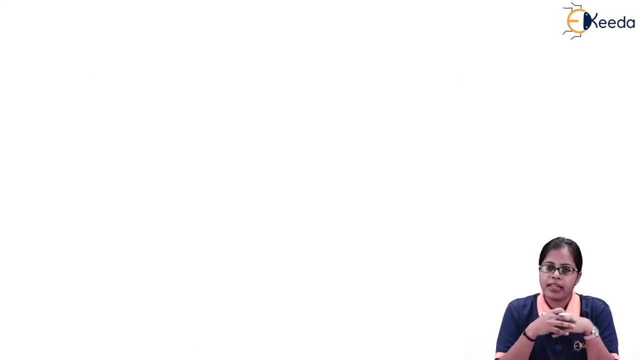 dipole moment. so this is what we talked about: electric dipole. so, as i said, to talk about dielectric material, the most important parameter is: what do you mean by an electric dipole? so once the electric dipole is formed, we talk about dielectric material. as i said, dielectric material are nothing but insulators. 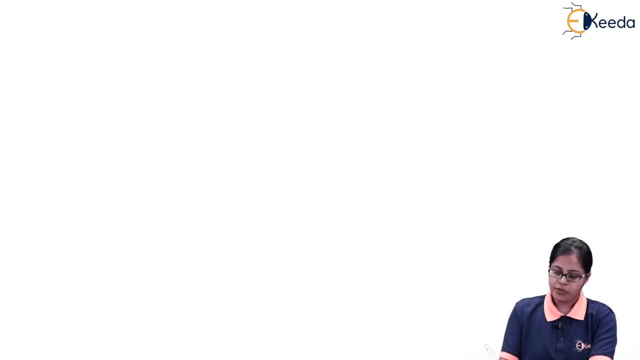 or they have no free charges present in them. so whenever we talk about dielectric material, dielectric material is going to be considered as insulating material, or we can say non-conducting material, firstly. secondly, we can say: as they are insulating material, it will have no free charges in them. 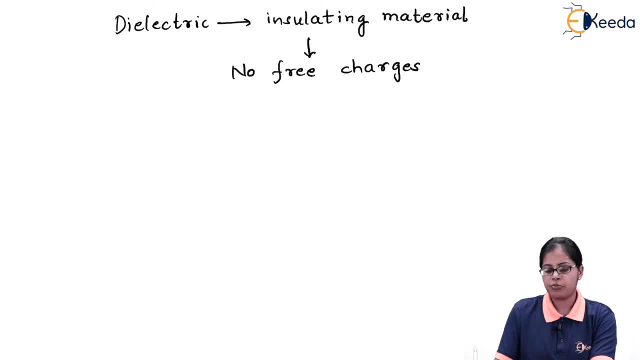 so if there are no free charges present in them, the material is going to be insulating or it will be considered as dielectric. now, depending upon whether a material consists of electric dipole or whether it has no electric dipole, we can classify the dielectric materials into two types. 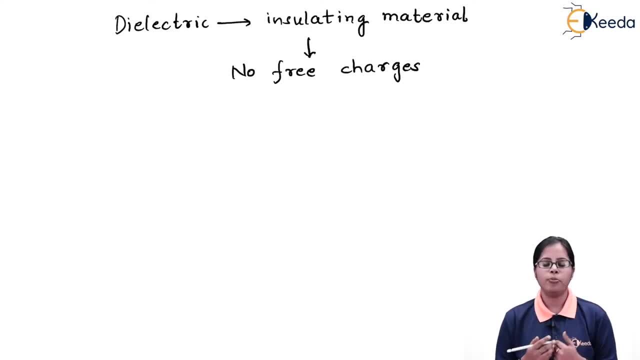 one is called as polar molecule and another one is called as non-polar molecule. so once we come to the classification of dielectric material, so this dielectric material can be classified into two types: one we can consider as polar molecule and the second one we can consider as non-polar molecule. 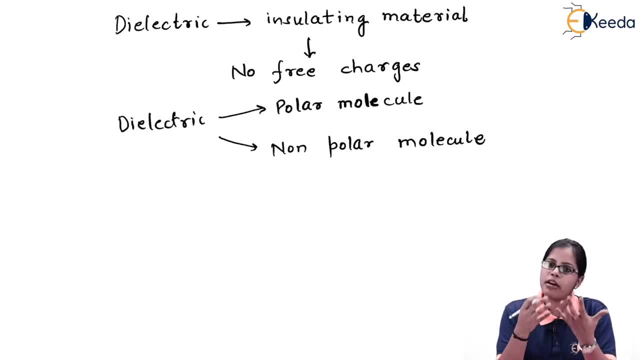 so when we say dielectric material will consist of either polar molecule or non-polar molecule, now obviously question arises that what do you mean by polar molecule? what do you mean by non-polar molecule when we say: if i have a material which is consisting of electric dipole permanently? 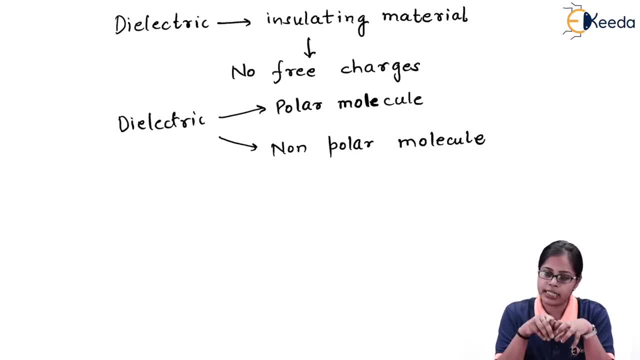 or initially it has the presence of electric dipole in it, that molecule will be classified as polar molecule. but if i have a material in which initially there is no electric dipole present, or if there is an absence of electric dipole in the material, that is considered to be non-polar, 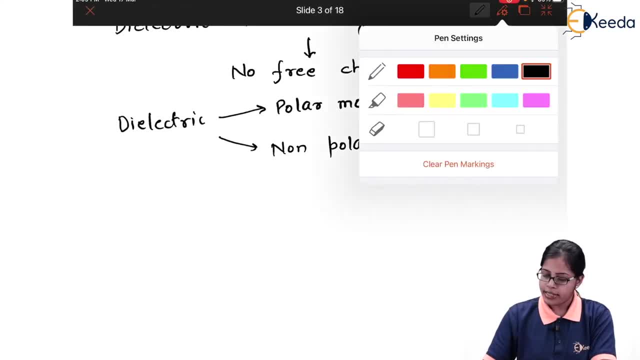 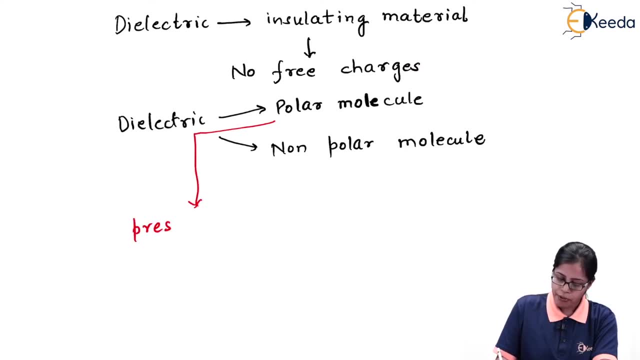 molecule. so when we talk about polar molecule, we can say that polar molecule is considered to have presence of electric dipole- the one which we have talked about in the previous slides- and when we say non-polar molecule, it has the absence of electric dipole. so if we have the presence of 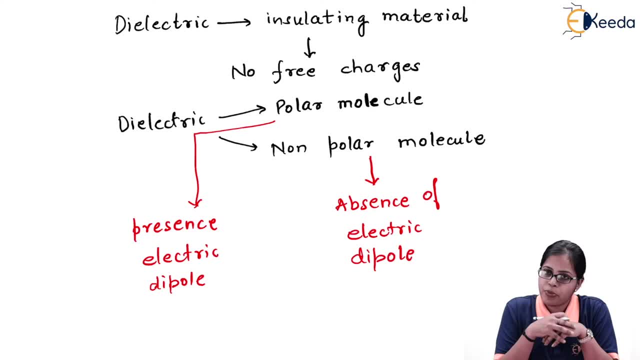 of electric dipole in the material, it is going to be considered as polar molecule. but if we have an absence of electric dipole, it is going to be non-polar molecule. so any dielectric material can be made up of either polar molecule or a non-polar molecule, depending upon whether it 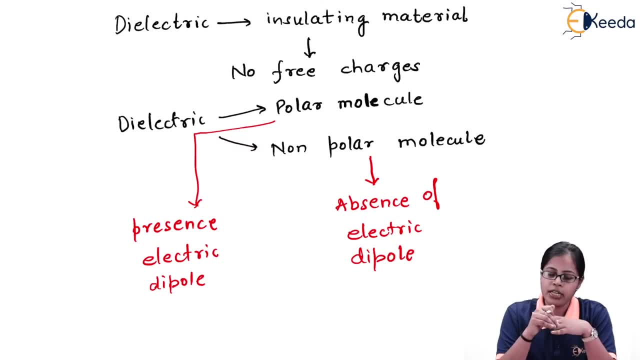 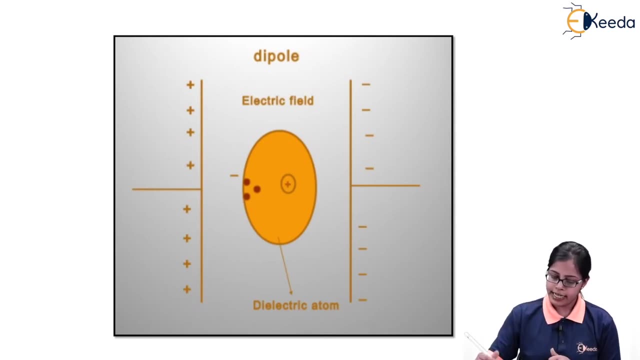 has a presence of electric dipole or absence of electric dipole. so when we talk about any dielectric material, i said they have no availability of free charges. so in this case, if you look at this particular diagram, it indicates that i have two metal plates. this one, 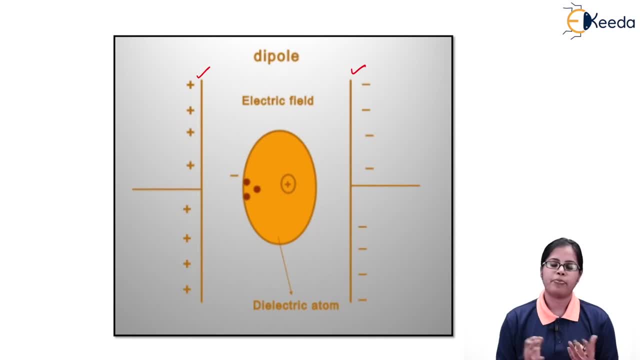 and a second, and these two metal plates are deposited by opposite charges, like these are positive charges, and on this plate we have deposition of negative charges, and in between this particular two plates we have the presence of dielectric material. obviously, if there is a presence of dielectric, 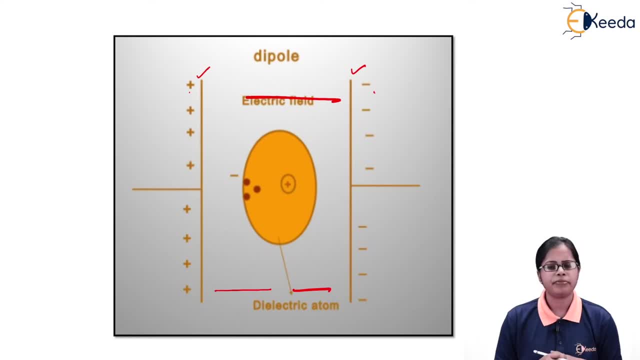 material, there will be presence of dielectric atom in it. now, when we say dielectric atom, it is either they can be polar molecule or non-polar, but simply please keep in mind that dielectric is going to be a insulating material or a non-conducting material. 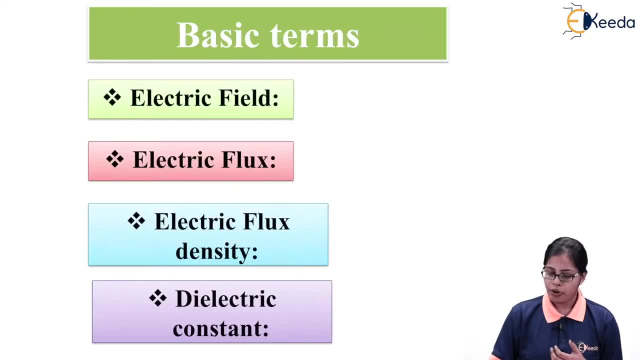 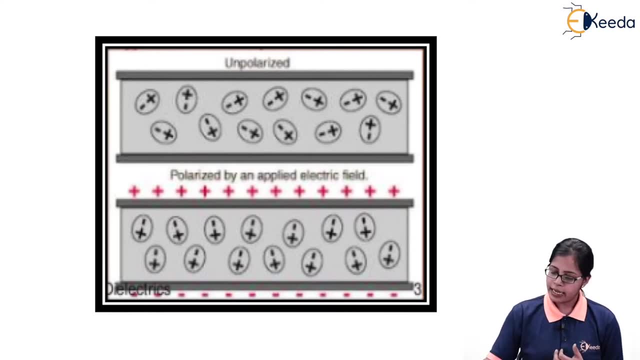 next is the process of which is called as polarization. when we talk about polarization, like normally, if i draw a diagram like this, like negative with a positive sign and drawn in a shape like this, this indicates electric dipole, that is, two equal and opposite charges separated by finite distance. so whenever 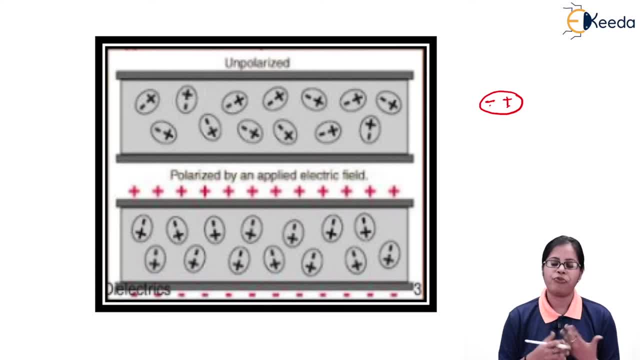 we look at a diagrammatical representation of electric dipole. it looks like this: like if i draw a shape like this with a negative and positive, this indicates the electric dipole now in the first diagram. as you can see, in the first diagram we have many electric dipoles present. 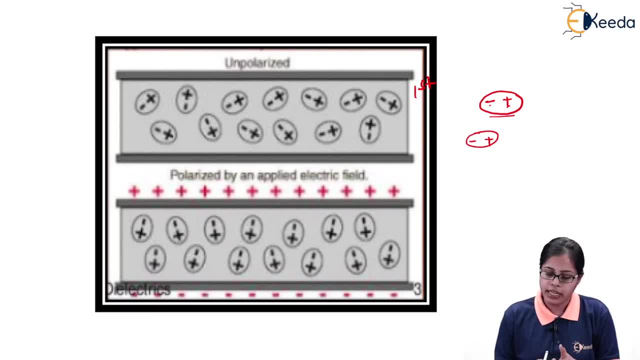 so if i have many electric dipoles present in it, that means they are considered to be polar molecule, but problem is that they are randomly oriented, they don't have proper orientation. So if the electric dipoles like this is indicating one electric dipole, this is indicating the second electric dipole. this indicates the third electric. 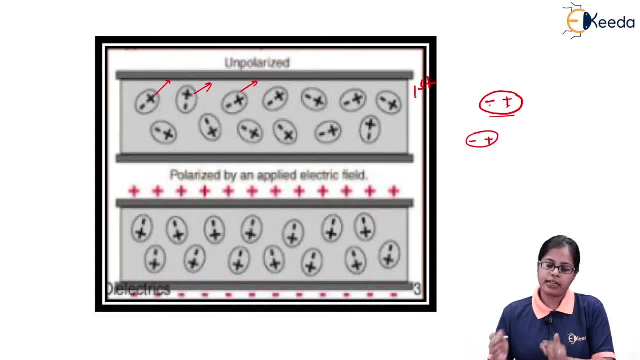 dipole. So I have many electric dipoles present in that dielectric material, but as they are randomly oriented, So if they are considered to be randomly oriented they are considered to be unpolarized. But if we consider another dielectric material and if that dielectric material is, 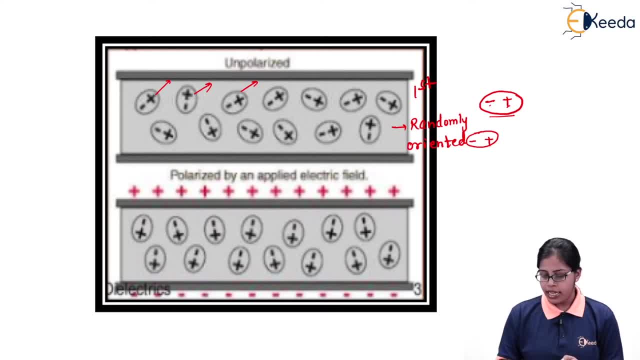 subjected to external electric field and if I get alignment of all the electric dipoles means the orientation of electric dipoles is properly in line. in that case the material is said to be polarized. That means, if I have material that is, 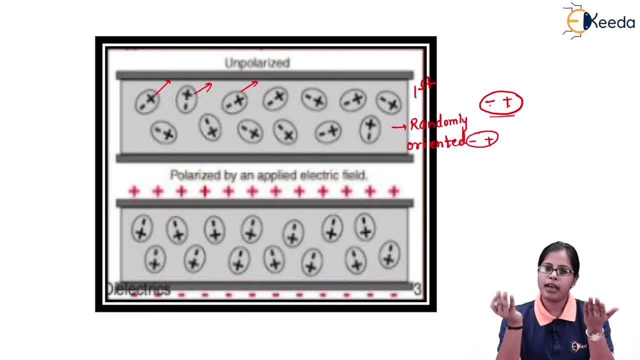 dielectric material in which electric dipoles are randomly oriented, then those materials are considered to be unpolarized. But if I have dielectric material having electric dipoles aligned in a perfect direction, in a certain direction, that is going to be polarized. That 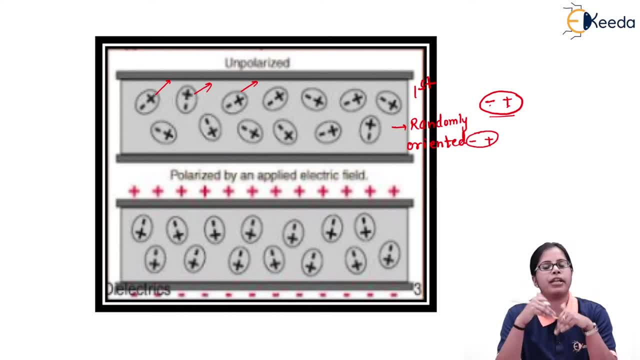 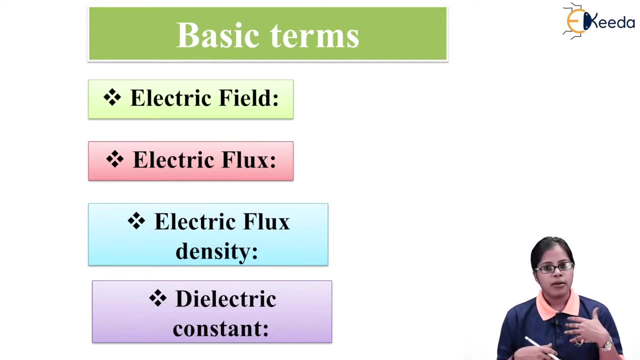 means I will either get an unpolarized material or a polarized material depending upon a certain factor. Let's look at the following. Let's look about: at what factor does it depend on? Next is, before starting with the concept of polarization, that is, a process of polarizing or aligning the dipoles in a material, we are going 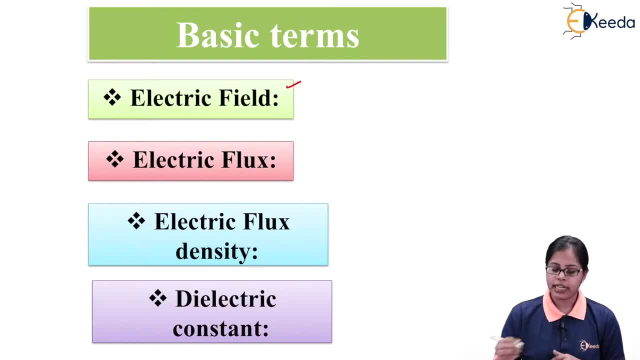 to talk about the basic terms. That is, first, is electric field. What do you mean by electric field? Why do we require electric field, Like whenever we talk about electric charges, whatever be the type of electric charge, Whether we talk about positive electric charge, whether we talk about negative electric charge, every electric charge- 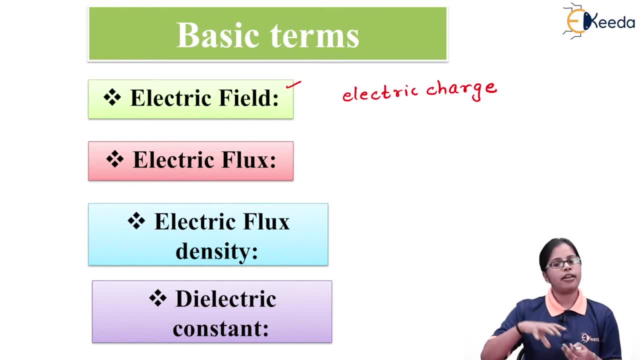 have a surrounding around them and the space surrounding the electric charge will be given by electric field. That means every electric charge will be surrounded by a space in which I can either experience a force of attraction or repulsion. If I consider the electric field, I also need a space around the electric charge, or negative electric charge. 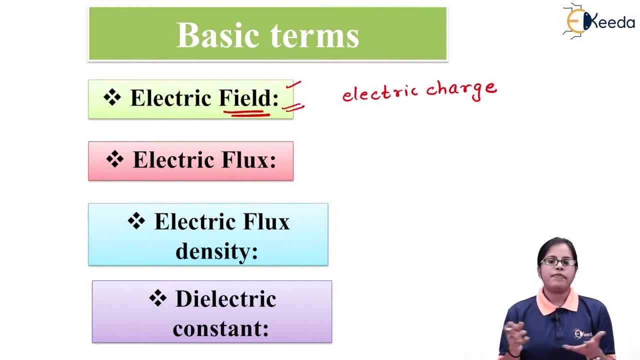 The electric fl? rush was referred to as electric field. Let's first könnten include a specific electric flux as well. Any given electric flux will 나는 also be a unit element. That is, a given electric flux is a unit element. All electric charges have general electric flux or electric flux will have a specific electric flux element. 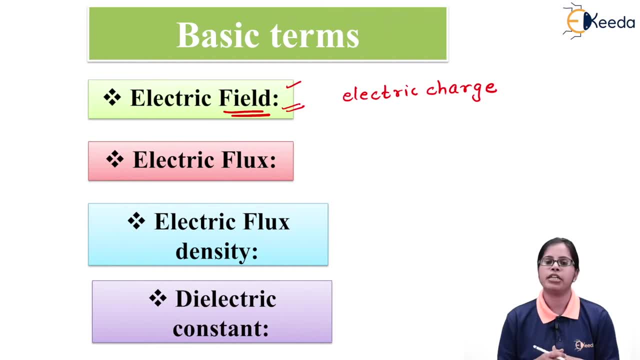 Let's assume that electric earth will have a specific flux and electric fluxダn six delta ddn will alias reach a specific electric flux. but it doesn't mean that electric flux is the strength of electric flux, lavender or 29th electric flux. You can easily say, of course, this vectorious and varying electric flux. 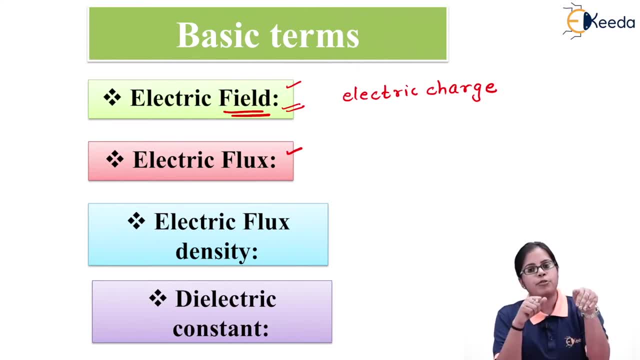 whenever we consider electric charges, the space surrounding them is called as electric field. this is like we have kept that concept in mind, but if i want to draw that there is a presence of electric field around the electric charge, we are going to draw it diagrammatically using. 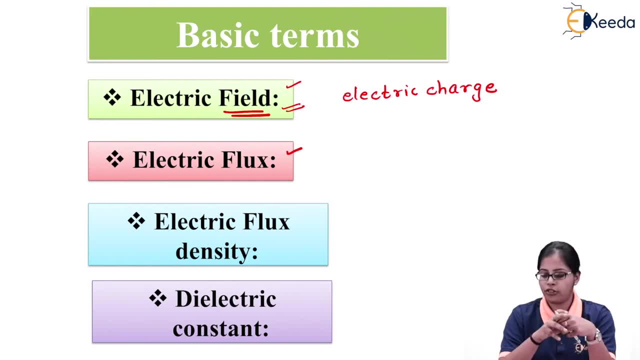 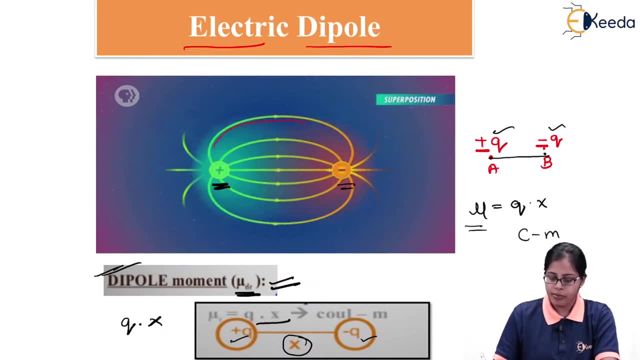 lines of forces, which is called as electric lines of forces. as i have shown in the previous diagram, this lines are nothing but indicating the electric lines of forces, which are all originating from positive charge and they all are terminating at a negative charge. so what is this electric lines of forces indicating? they are indicating the presence. 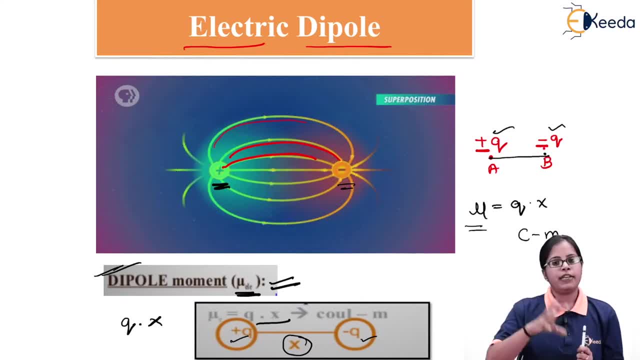 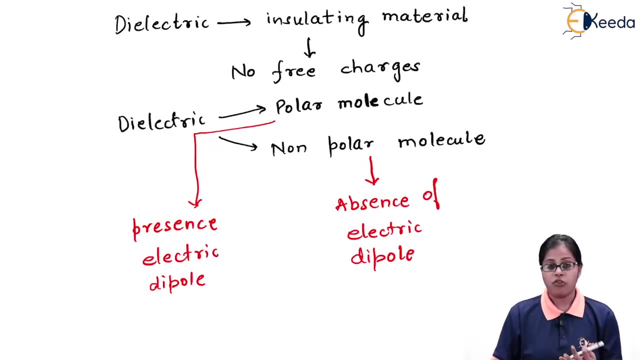 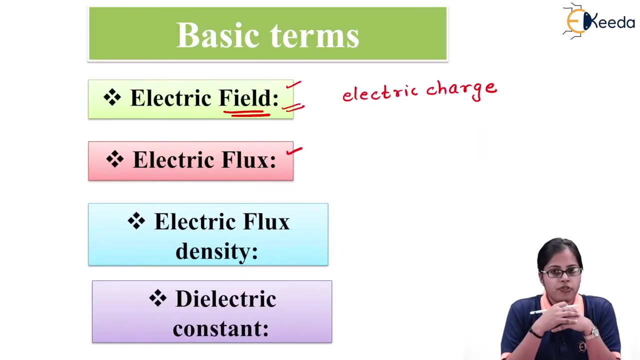 of electric field around the charges. that means if we want to show that electric field is present in a certain area, then we are going to make use of electric lines of forces to show diagrammatically that there is a presence of electric field. so obviously, electric lines of forces are- is an important term. so when we talk about electric lines of forces, 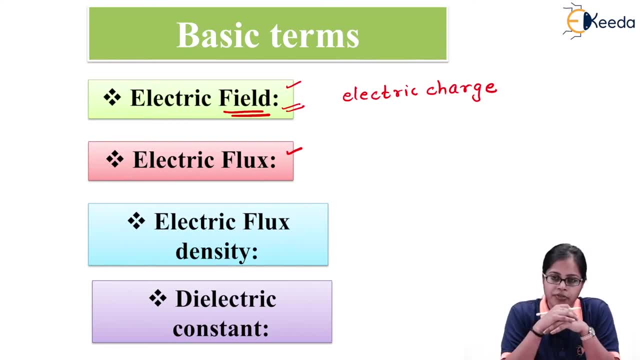 what is going to give or lead to the concept of electric flux. suppose there are certain lines of forces passing through this region and if i calculate the number of lines of forces passing through a cross-sectional area? so i have calculated the lines of forces which are passing through a cross-sectional area. 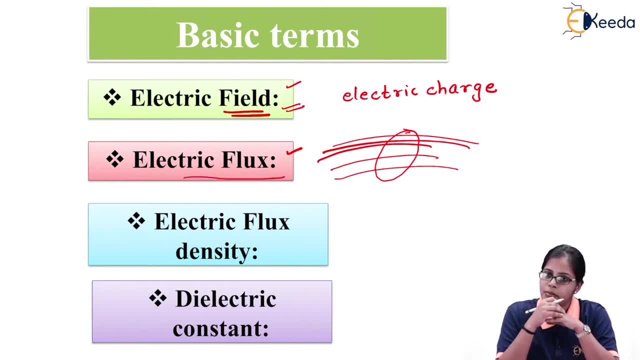 that number is called as electric flux, but i have one more term, that is electric flux density. so what is the difference between electric flux and the electric flux density i said over here? i am calculating the number of lines of forces passing through a cross-sectional area. but when we talk about electric lines of forces passing through a cross-sectional 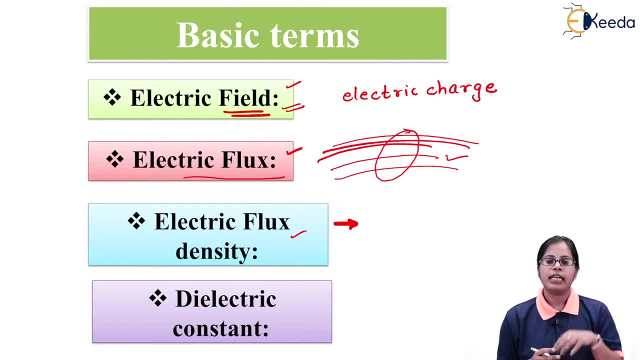 area. that is called as electric flux density. in that case we talk about the number of lines of forces which are passing normally per unit cross-sectional area. that is called as electric flux density. that means there is like peculiar difference between the two terms. when i say electric flux, it is the number of lines of forces passing through a cross-sectional area. 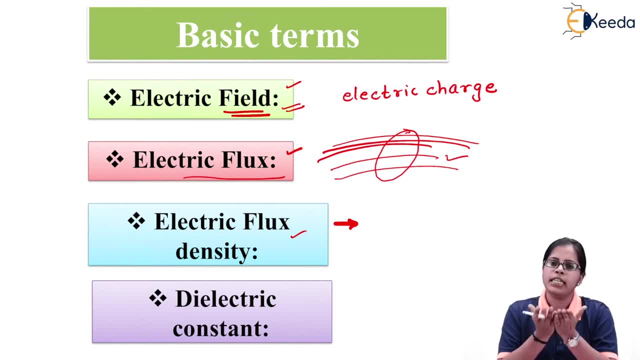 just number of lines of forces passing through any cross-sectional area. so electric flux density will be considered as electric flux. but when we consider electric flux density we need to talk about the number of lines of forces which are passing normally per unit area, or you can say normally per unit cross-sectional area. so in that case we call that number of 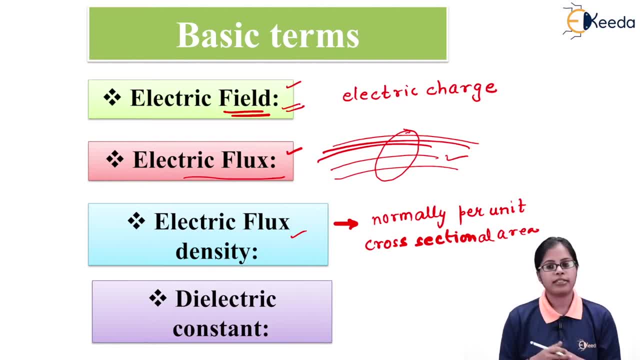 lines of forces which are passing normally per unit area. that is considered to be electric flux density. now, obviously, if you are not aware of the term normally, normally means they are passing in a perpendicular manner. so if they are passing in a perpendicular manner through a certain unit cross-sectional area, so that number of lines is going to give. 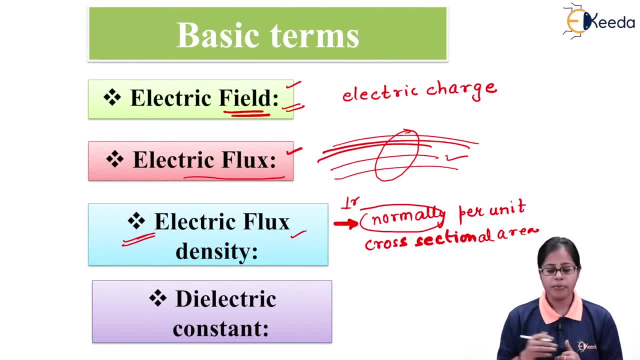 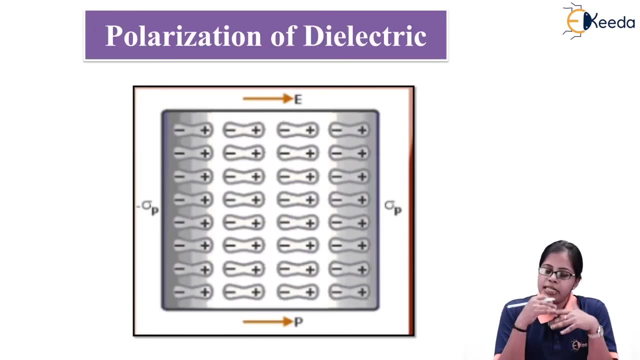 me a quantity called as electric flux density. next, when we talk about dielectric constant, these are the terms which are related to the concept of electric flux density. so electric flux density, where you say that it is a material being offensive, such that you can also consider dielectric current as electric flux density. as for supposing that, aistically, the length 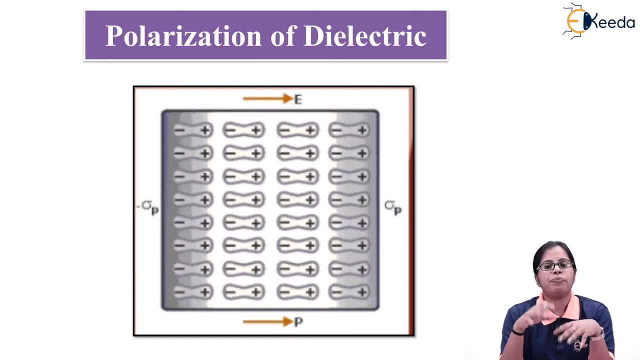 of the coir is multiplied after, which is given as electric gross response, right? so for example, if we use the term electric flux density, we can take Engine voltage. So here I say electric flux density, here you need a certain amount of working resistAn ��50. 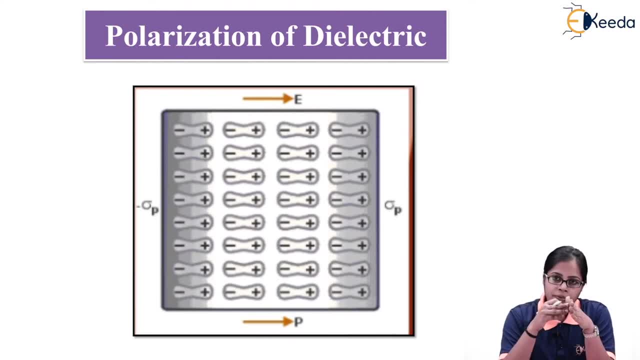 gider and the dipoles which were randomly oriented, they all are going to get oriented in the direction of electric field. so if the dipoles get oriented in the direction of electric field or the external electric field, we say that materials are getting polarized. so whenever we talk about the polarization, 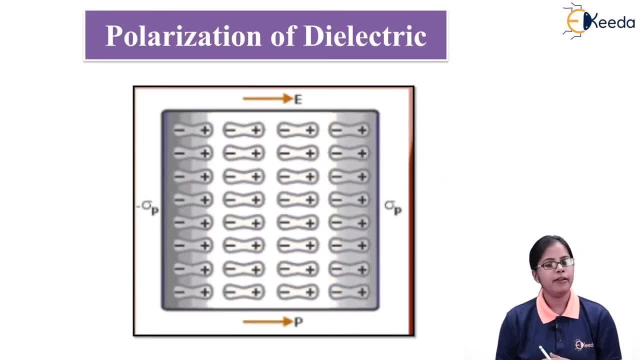 of dielectric material or whenever we want to polarize a material. suppose if i took a dielectric material. in that dielectric material, in the absence of electric field the dipoles are randomly oriented. but as soon as i take the dielectric material and subject it to an external electric 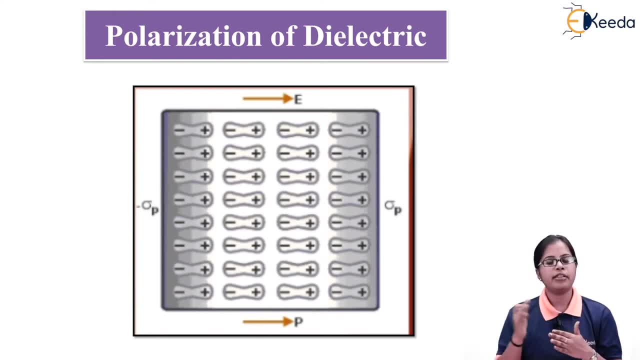 field, all the dipoles will start getting oriented in the direction of electric field. so that means what? that there is a certain effect of the external electric field on the dipoles which are present in the dielectric material. so this transition, that is, in the absence of electric field, that is, if i have no external 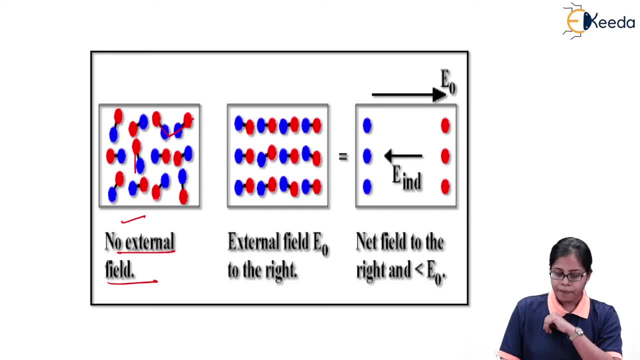 electric field. these are representing dipoles, so those dipoles are randomly oriented. so you have to keep in mind that suppose if i have a dielectric material and suppose this is polar material, so i have a polar dielectric material if i say it is a polar dielectric material. 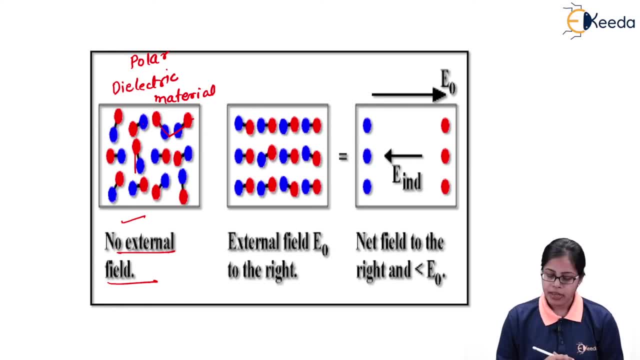 means it already has a presence of electric dipole. but, as you can see, there is a presence of electric dipole, but they are randomly oriented. this has some other orientation. this has some other orientation. so we can say that i have considered a dielectric material which is 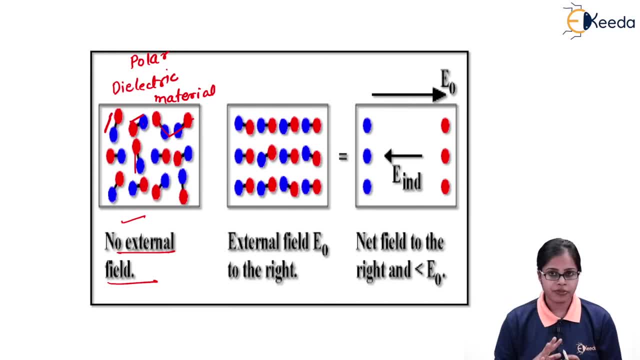 polar. polar means it will have a presence of dipole. but in the absence of external electric field the dipoles are randomly oriented. so if they are randomly oriented the effect is going to be a dipole get nullified and there will be no polarization. but if I subject that same material to an 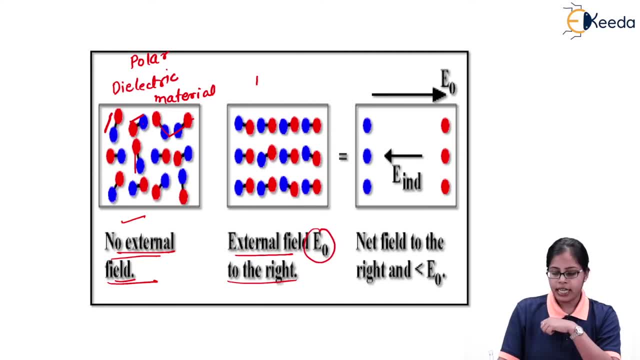 external electric field E0. this external electric field E0 is directed in the right hand side direction. so what is happening in this case is that the dipoles are getting oriented or aligned in the direction of electric field. that means there is an effect of external 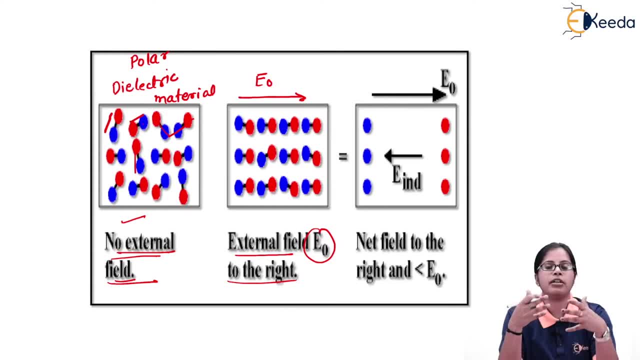 electric field on the polar molecule or the polar dielectric material. so if the polar dielectric material in absence of electric field will have random orientation of dipoles, but if we subject it to external electric field it will have proper alignment in the direction of external electric field. so if the dipoles get properly aligned in the direction 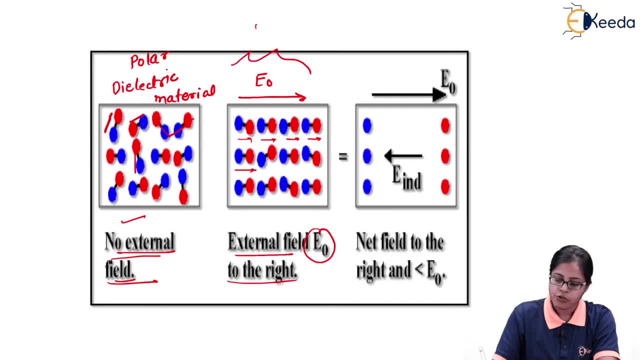 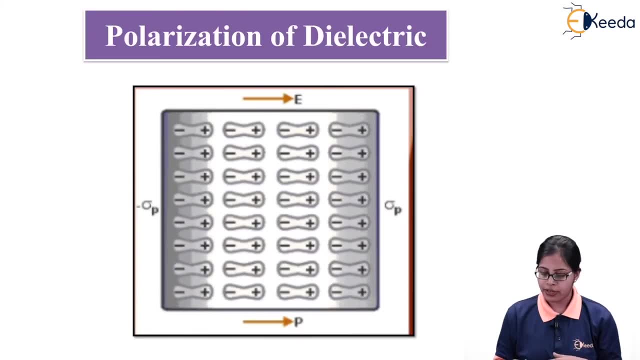 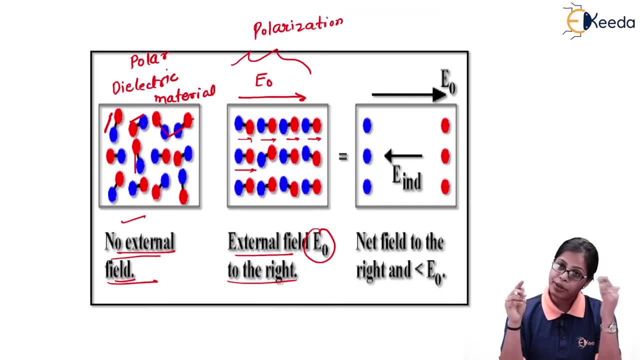 of external electric field, we call that phenomena to be polarized. So when we talk about the polarization of dielectric material, this is nothing but the alignment of dipoles which were previously randomly oriented, and they are getting aligned in the direction of the applied external electric field. so if the external electric field is, 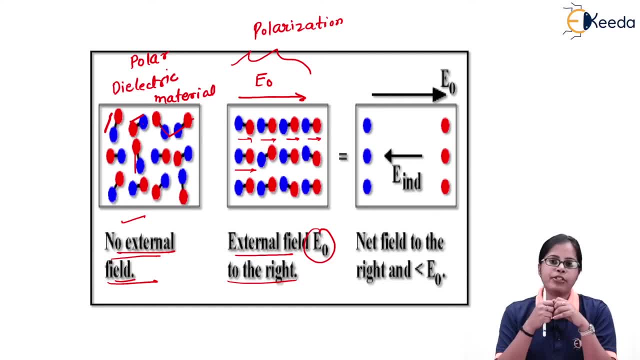 pointing towards the right, the alignment will be towards right. if the external electric field is towards left, so the alignment of the dipoles will be towards left. so this alignment of the electric dipoles in a dielectric material is called as polarization. now, as soon as the dipoles get 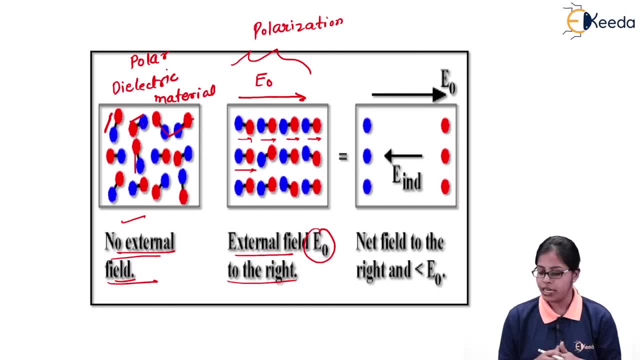 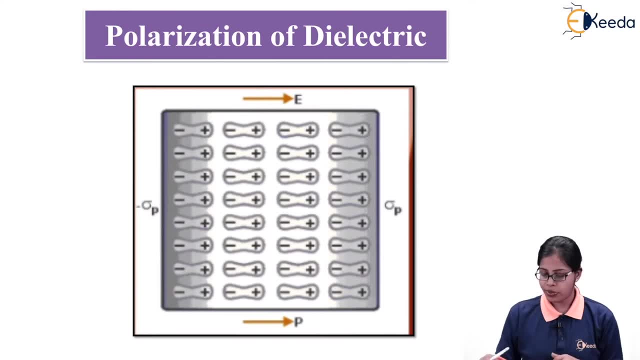 aligned in a certain direction of the external electric field. we get induced electric field inside the dielectric material. now, as you can see in this particular diagram, we have all the dipoles which are aligned in a certain direction. but if you look at the direction of external electric field, the direction of external, 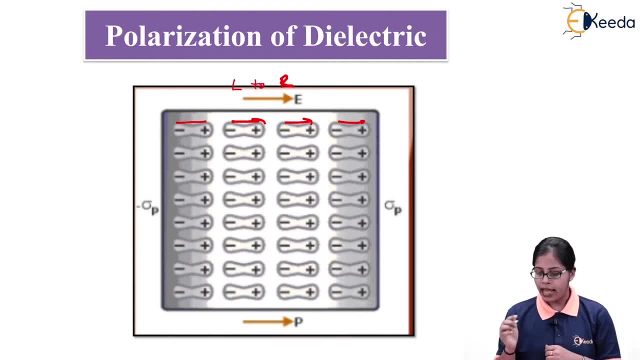 electric field is pointing from left to right, and the dipoles, that is negative, and the positive charge, separated by certain distance, they all are getting in aligned in the direction of external electric field, keeping in mind that the positive charged or negative charged electric field charges are going to be in the direction of electric field. so as soon as I 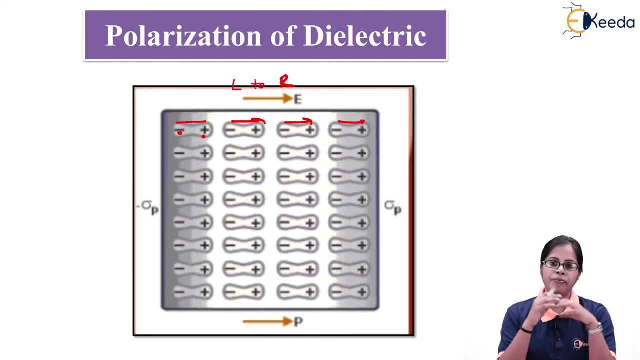 subject: this dielectric material to external electric field. all the dipoles are getting aligned in the direction of external electric field. now what is going to happen internally is that this positive charges are going to cancel out. with this negative charges means they are going to nullify each other's effect. 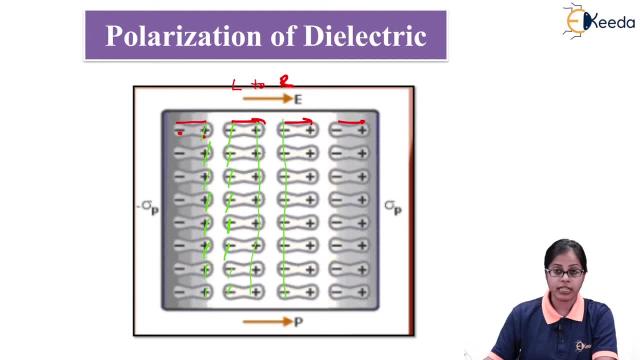 like this positive charge has going to nullify the effect with the negative charge. this positive charge will nullify the effect with this negative charge. so if you look at the internal charges of the dipoles, they are getting cancelled out with each other. so if I subject the dielectric material to an external 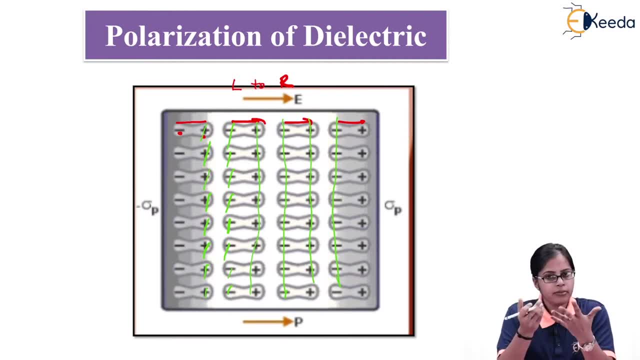 electric field. the dipoles are getting aligned, that's correct, but the charges which are present internally, they are getting can out with each other, leaving negative charges on the left-hand side and the positive charges on the right-hand side. that means the one surface of the 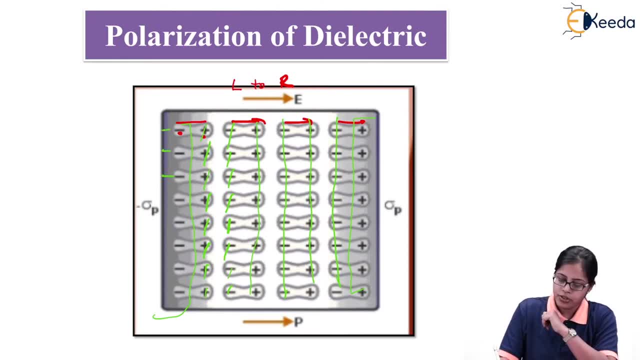 dielectric material will have negative charges on it and the one surface of the dielectric material will have positive charges on it, and all the internal charges are going to cancel out each other. but this is all going to happen after the polarization, after the alignment of the 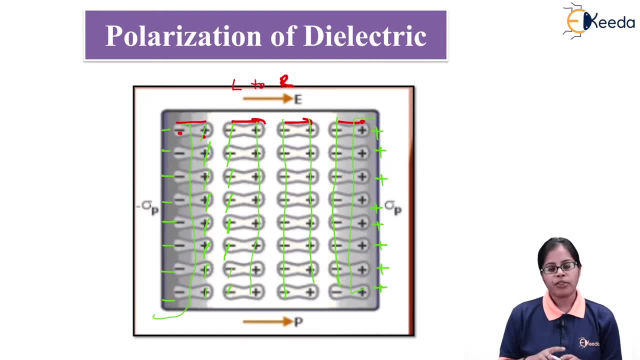 dipoles in the direction of external electric field. so once I get this particular concept, this is giving me a negative charge on one plate and positive equal number of positive charge on another plate, and I already had external electric field in this direction from left to right. so this is. 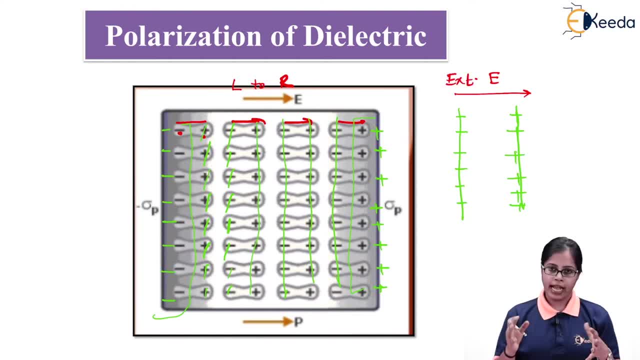 your external electric field pointing from left to right, and all the dipoles got aligned in the direction of external electric field by leaving or cancelling all the in between charges, leaving only negative charges on the left side of the material and positive charges on the right hand side. so if I look at the 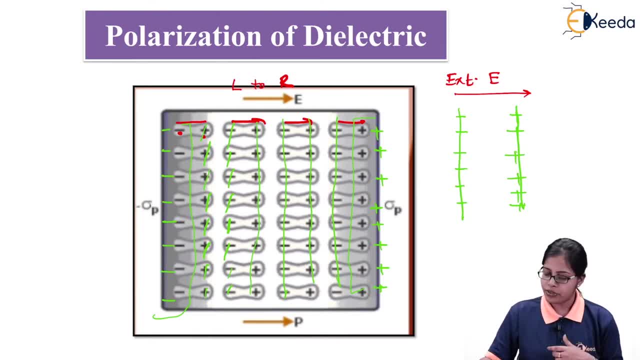 direction of electric field. in side the dielectric, it will be from positive to negative, because we have to keep in love in. the direction of electric field is always pointed from positive to negative. so the next or the new electric field which is getting indicated away here is nothing but the induced electric field. 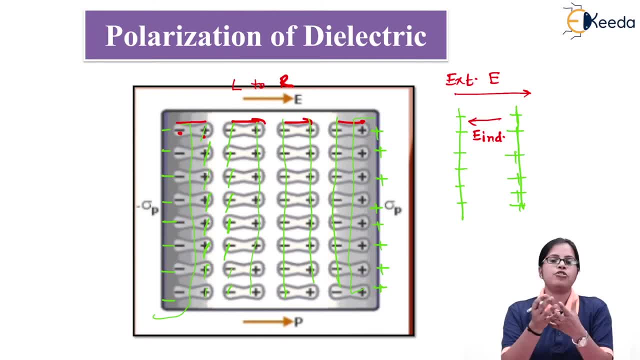 this induced electric field is nothing but induced due to the charges which are developed on. the plates have a negative charge on one plate and it equates to one plate and the positive charge. so due to this negative and positive charge of the dielectric material, i'm getting induced electric field pointing from right to left. so overall, if you look at the 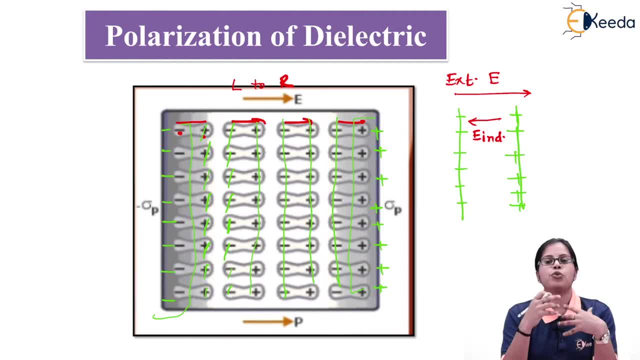 dielectric material. i have an external electric field due to which polarization of dielectric material is occurring and because of the cancellation of the charges present inside the material, i've been left with only two charges, one as negative, another one as positive, so that two set of charges on the two plates of the dielectric material leads to new electric. 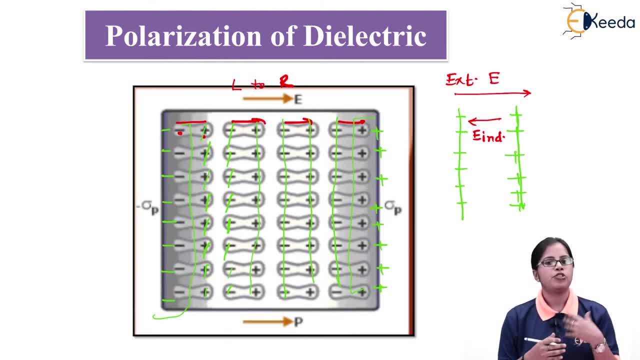 field which is the induced electric field inside the material. so we have overall two electric field. one is the external one, which is used for polarization, and the second one which is the induced electric field, both in the opposite directions. so the polarization of dielectric material leads to the production of electric dipoles. 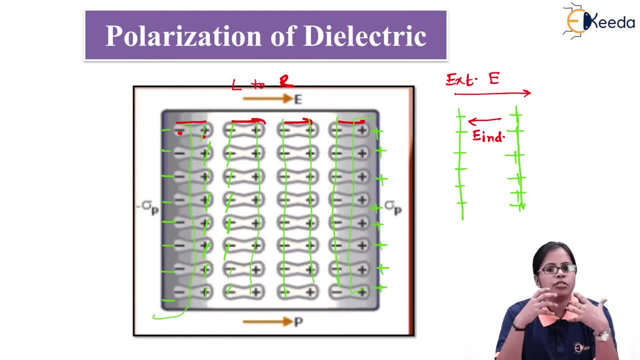 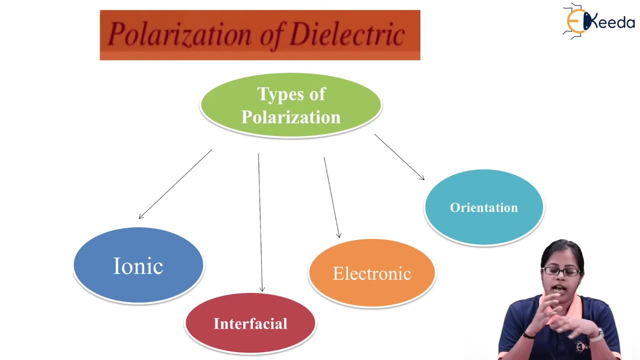 inside the dielectric material. so this process of production of electric dipoles inside the dielectric material is called as polarization. obviously, as we have understood that, what do you mean by polarization? that how a dielectric material, whether it is a polar material or a non-polar material, it can be polarized. so the polarization of dielectric material is called. 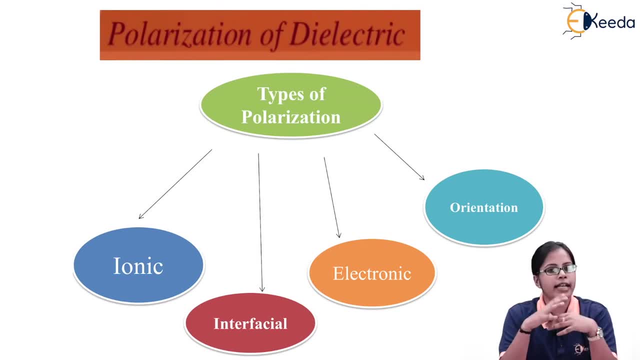 as polar Can we polarize? like, if you have a polar molecule it already has a dipole, so we can polarize the material easily. but if we have a non-polar molecule, we can even polarize that material, but the polarization required for non-polar material will be more as compared to the polar. 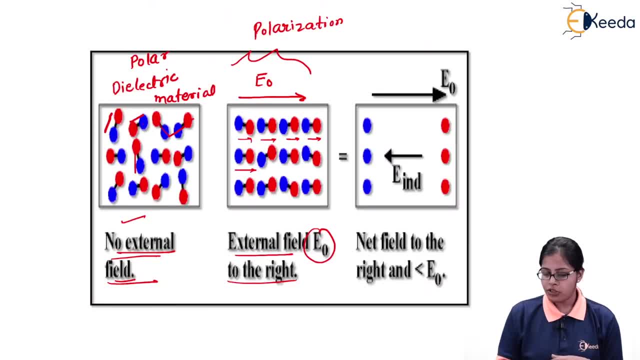 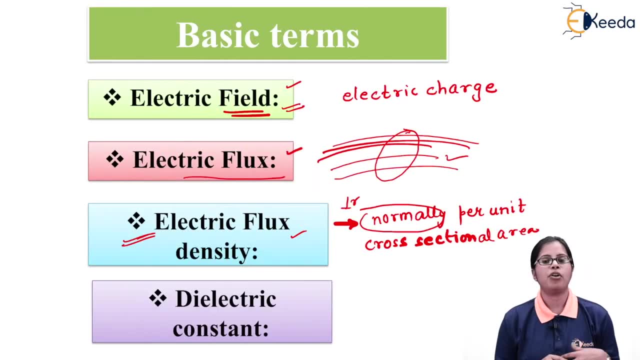 molecules. so when we talk about this polarization, there are certain more parameters which come into picture. that is, one is the concept called as dielectric electric constant. Now, when we talk about electric field, there is a parameter which is important when we talk about electric field, that is, we talk about the epsilon. Epsilon is nothing but called. 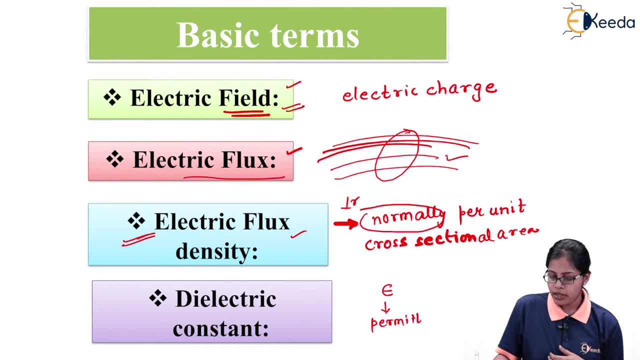 as permittivity. Now, whenever we take the ratios of permittivity, either in free space and if I take the permittivity in medium, like I can have a charge placed in free space or vacuum, in that case we are going to consider the permittivity of free space or vacuum. but if I place the charge in 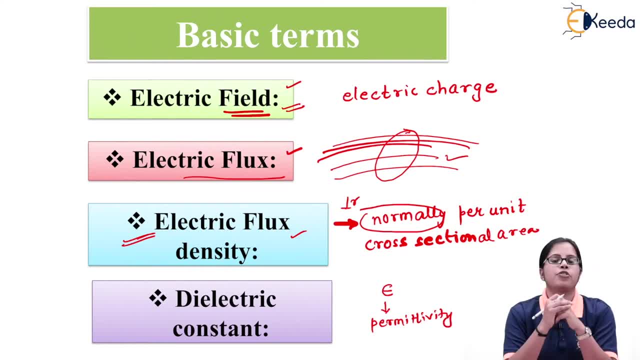 medium. we need to consider the permittivity of the medium. So we have two permittivities, that is, one is permittivity of free space or vacuum, when the charges are placed in free space or vacuum, and I have permittivity of medium when the charges are placed in medium. So these are the two permittivities which we are. 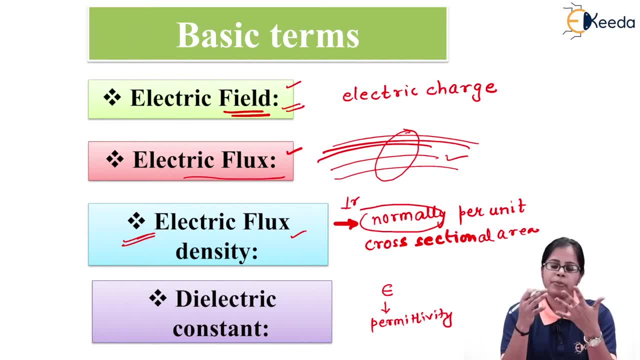 going to talk about and if I take the ratio of this permittivities, that is, permittivity of medium, to the permittivity of free space, that leads to the term called as relative permittivity or it is also called as dielectric constant. So, as I said, that we can either place the charges, 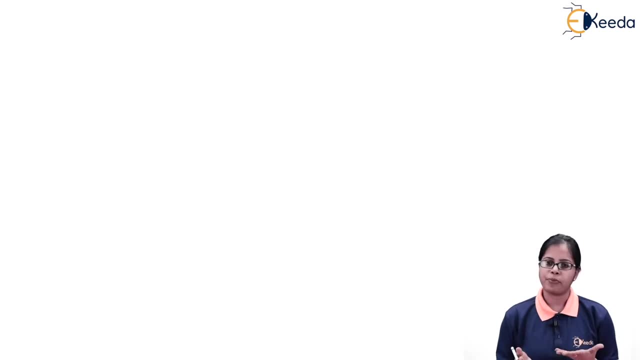 in medium or I can either place the electric charges in vacuum but accordingly we need to consider the permittivity. that if I place the charges in the medium, we are going to consider the permittivity of medium, but if I place the charges in vacuum we need to consider the. 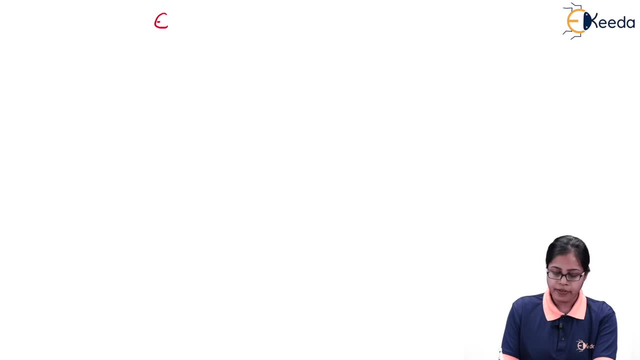 permittivity of vacuum. So there are going to be two permittivities. either you can write it as epsilon, the other one is written as epsilon naught. Epsilon is nothing but called as permittivity of medium, that is, when the charges are placed in medium. 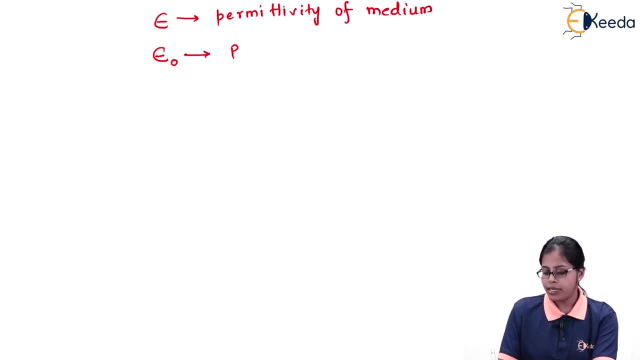 then we talk about epsilon, and when we say epsilon naught, it is considered to be the permittivity of free space or vacuum. So these are the two permittivities as they are same quantity if I take the ratio of epsilon upon epsilon naught, that is the permittivity of free space. 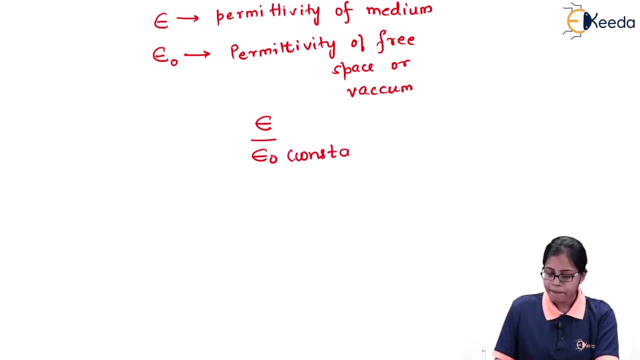 or vacuum is always constant. But when we talk about epsilon, epsilon keeps on changing with medium. if I keep on changing the medium, the epsilon value keeps on changing. so in that case epsilon has a variable value. So out of epsilon and epsilon naught, epsilon naught is completely constant because of permittivity. 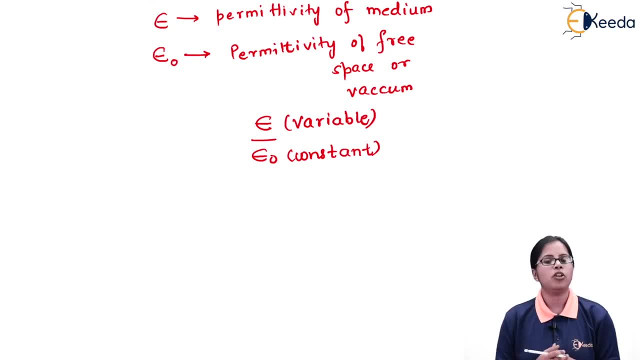 of free space is never going to change. but when we talk about epsilon, epsilon is related to medium, So it is going to change the permittivity of free space, So it is going to change the permittivity of free space. So it is going to change the permittivity of free space. 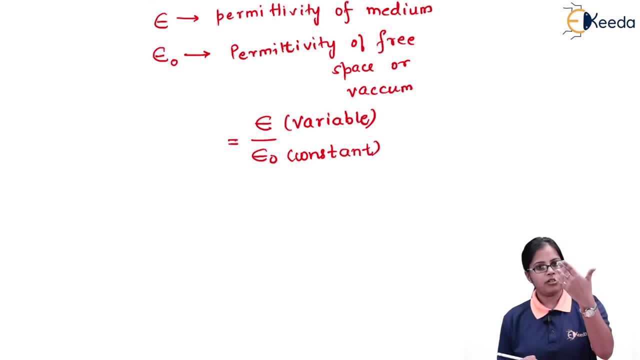 So if I have a term divided by same terms, that is, I am dividing two same terms, that is, permittivity by permittivity. Just the difference is one is in medium and the other one is in vacuum. One term is variable and the other one is constant. 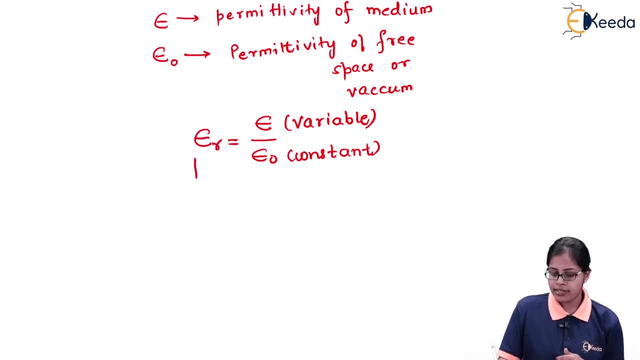 So I am going to get a permittivity term which is called as relative permittivity, or sometimes it is also written as dialectical permittivity. So, besides the p at the other side, this term is So, since it is only a definite form of permittivity, which is also written as faz syndrome. this 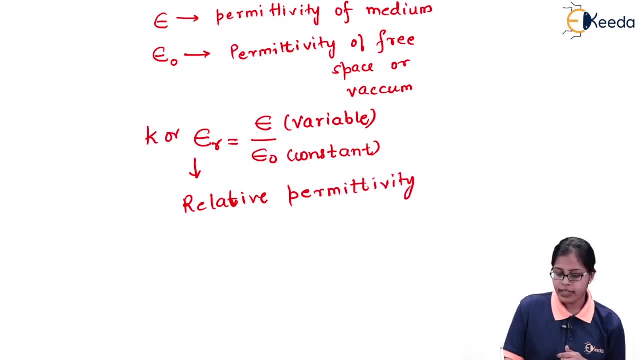 term has a unpatriotic form, but I am going to say as subtle form, that is Kendra Dirull's least: эту will darum sto où deciren. Or either you can write the relative permittivity, The bond, as the ratio of permittivity of medium to the permittivity of free space, of vacuum. 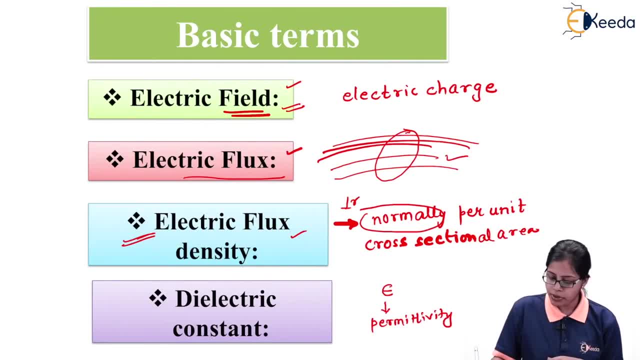 So when we say dielectric constant, dielectric constant is nothing but written as epsilon, as epsilon upon epsilon, not. Or you can write dielectric constant, So just taking the call k. So either we can call it as k, that is dielectric constant, or you can even term that ratio. 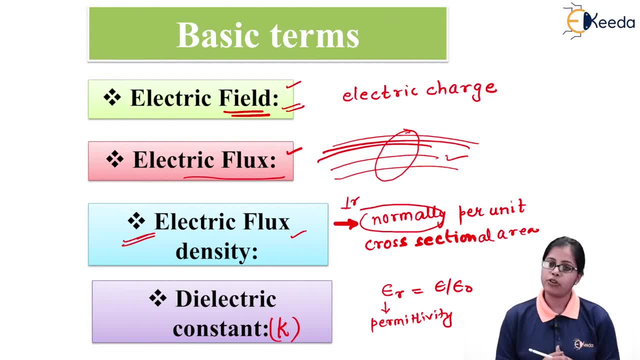 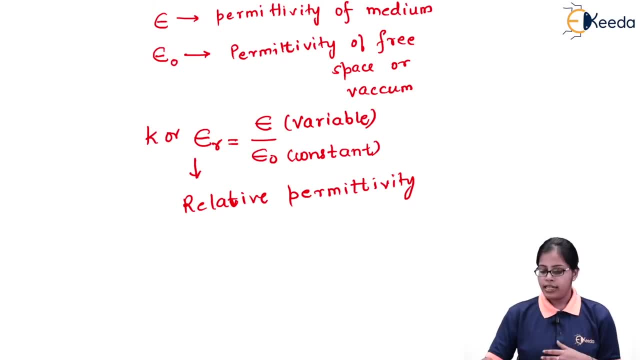 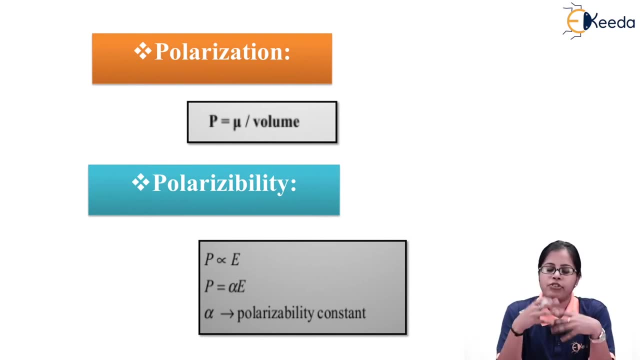 as relative permittivity. that is denoted by epsilon r. So this is how you define the term dielectric constant. Next is when we talk about polarization, as I said, whenever we are trying to induce electric dipole in a molecule or in a dielectric material, that phenomenon is called. 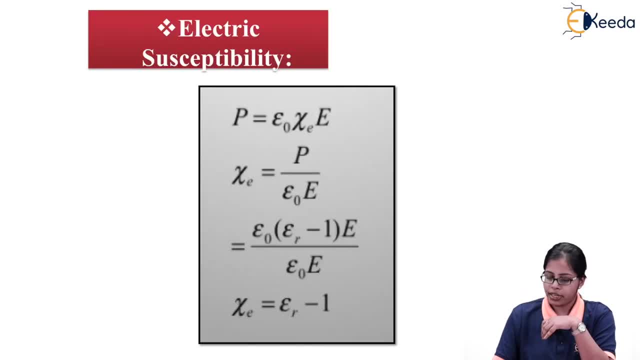 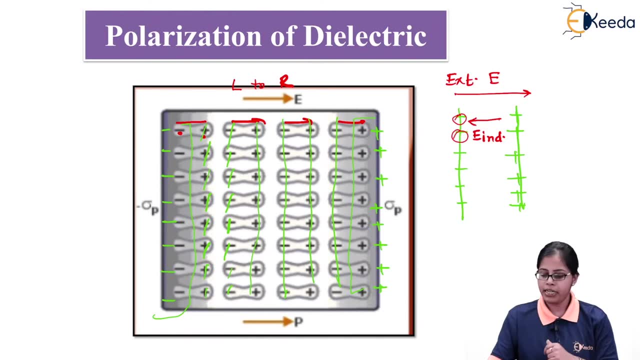 as polarization. So the induced dipole moment, like, if you can see in the diagram, we have induced the dipole moment. that is, we have induced negative charges on the left plate and positive charges. they are obviously separated by a certain distance between the plates, So we have induced dipoles. now, when we are inducing dipole, we are going to talk about a 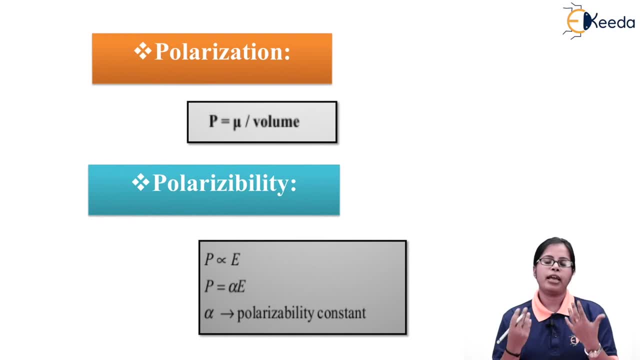 term called as polarization, like how much dipole moment is getting induced per unit volume of the material, is going to be called as polarization. So mu is indicating the dipole moment or, to be more specific, we can say it as induced dipole moment. So if I calculate the magnitude of 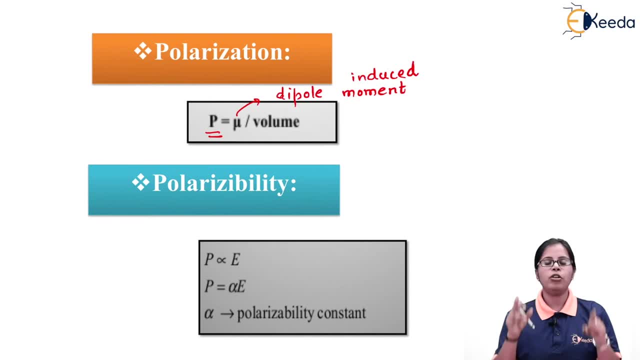 induced dipole moment per unit volume of the whole material of the dielectric, then that leads to the concept of polarization. Like if I say the induced dipole moment is more per unit volume than the polarization is more, If we say the dipole moment induced is less per unit volume, then the polarization will be less. 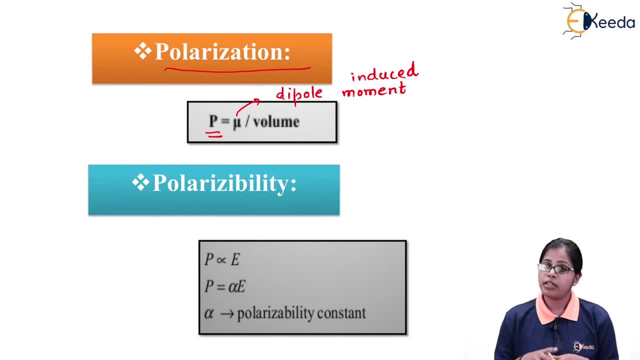 So the polarization material will depend upon the dipole moment which is getting induced in a certain volume. So for a certain volume, if the number of dipole moment induced is more, we can say the polarization is more for a certain volume of the number of molecules or number of dipole moments induced is. 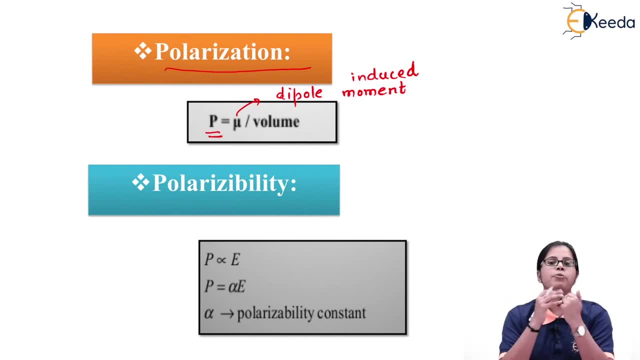 less than the polarization is less. So if we want to talk about polarization, it is nothing but the number of induced dipole moment per unit volume. Next is when we talk about polarizability. as I said, induced dipole moment per unit volume gives me polarization. but if we talk about polarization, 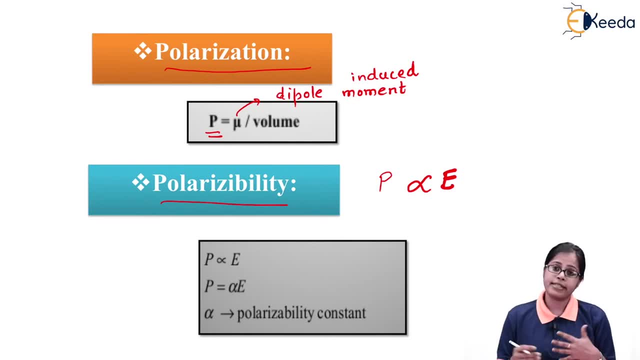 it is proportional to E. Why I consider polarization proportional to E? because polarization of any dielectric material depends upon the subjected external electric field. So if the dielectric material is subjected to high external electric field, the polarization will be more, That is more dipole moment will be induced. But if a dielectric material is subjected to 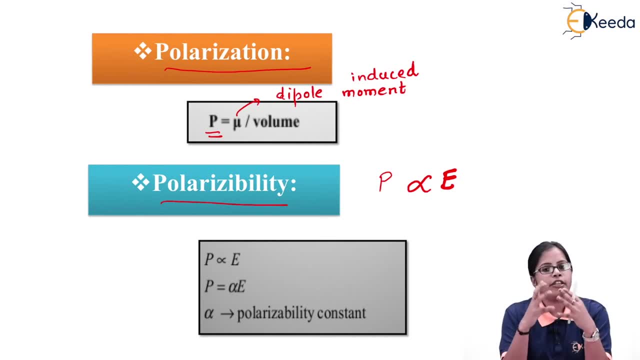 low external electric field, then the induced dipole moment will be less and the polarization will be less. That means indirectly can we say that polarization depends on induced dipole moment. Induced dipole moment depends on the external electric field. So indirectly we can say that the polarization is. 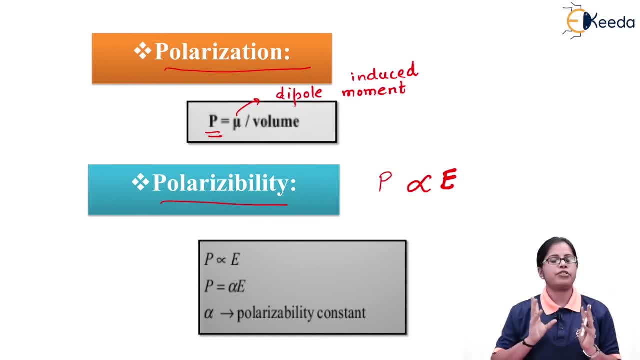 dependent on external electric field. That is, if the external electric field is more, I will have more induced dipole moment. that is more polarizability. But if we have lesser or low external electric field, we can say that that we have low induced dipole moment and low polarizability Means. polarizability of any dielectric material depends upon the magnitude of the external electric field, whether it is a strong electric field or whether it is a weak external electric field. That is why it is directly proportional to the strength of the external electric field. If the strength is strong. 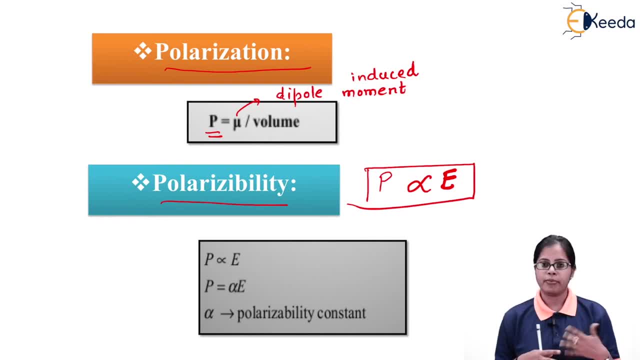 more will be the polarizability. If the strength is weak, the polarizability will be less. So, if we write the equation as p directly proportional to e, as we are already aware that whenever we write polarizability proportional to e or any term proportional to something, If we remove 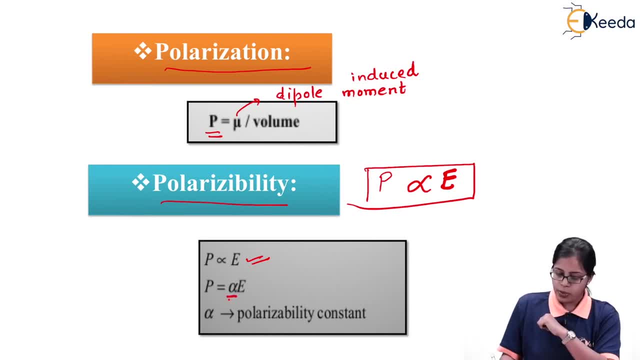 proportionality sign, we need to put a constant. Now, in this case we are getting, alpha has a constant. this alpha is nothing but called as polarizability constant. so there are two terms which are important in terms of polarization. one is the term polarization and the second is 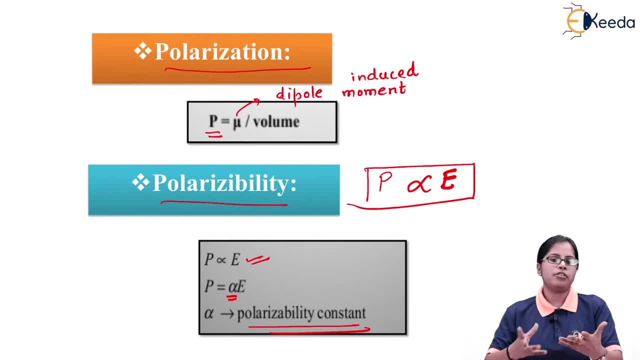 polarizability, which is entirely dependent on the strength of the external electric field. if the external electric field is strong, the polarizability of the material will be more, and if the strength of the external electric field is less or weak, the polarizability will be weak. 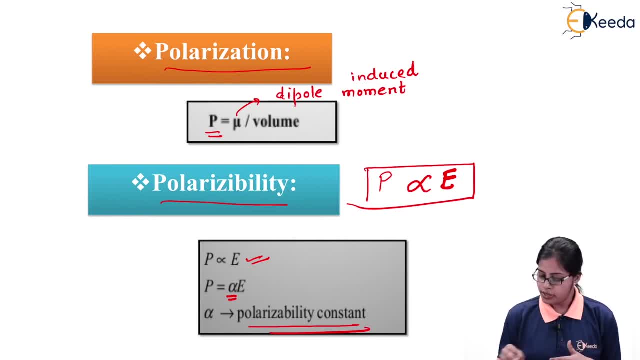 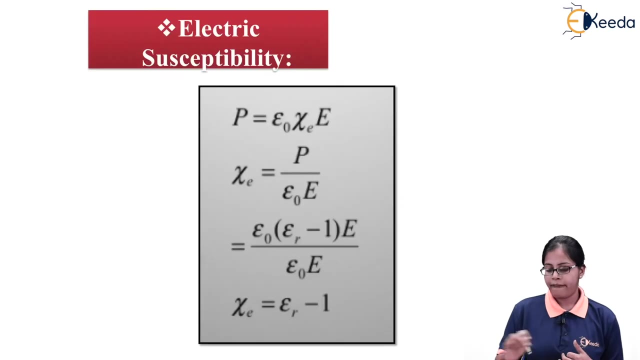 so we can say that they both are directly proportional to each other. so this indicates that p indicates polarizability and e indicates the external electric field. next is electric susceptibility. now, what do you mean by electrical susceptibility? is that whenever we talk about the polarization or polarizability relation with electrical 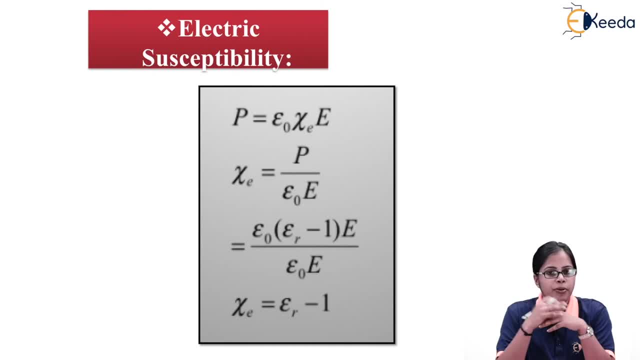 field intensity. in that case i said they are both proportional to each other. if i want to get that measure of polarization of any material and how much the material is getting polarized with the subjection to the external electric field, that measure of how much the material 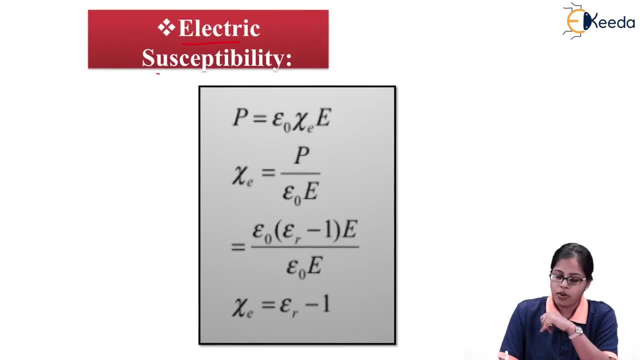 is getting polarized will be given by the property called as electric susceptibility. so we can say that electric susceptibility depends upon, or it is going to give me the measure of how much the material is getting polarized, or how much material is going to undergo polarization, depending upon the subjection to the external electric field. that measure of polarizability, 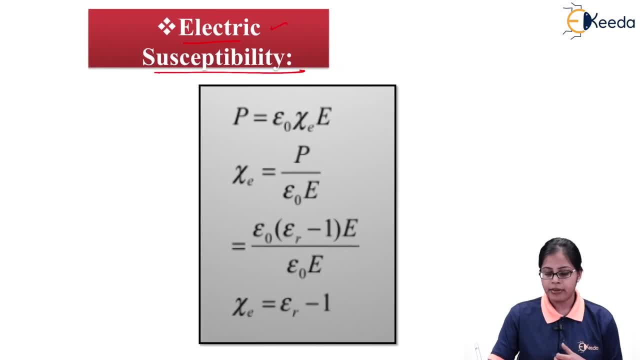 of the material is called as, or given by term, called as, electric susceptibility. in this particular term, p indicates polarizability, e indicates the external electric field and, as i said, these two terms, that is, polarizability and external electric field, the measure of how much the material is getting. 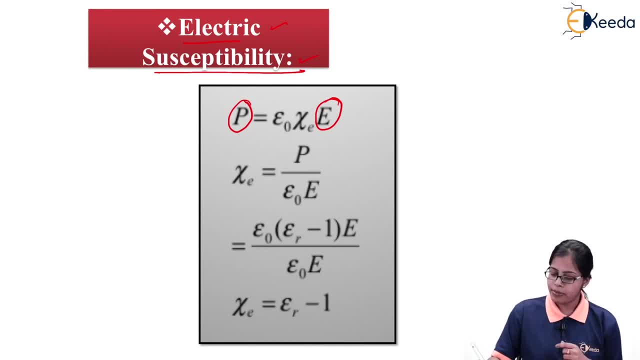 polarized, is dependent on the term called as susceptibility. so this chi or this term indicates the electric susceptibility. so if we want to get electric susceptibility, so mathematically this is the equation which we make up. but physical term wise, we can say that the measure of how much the material is getting, 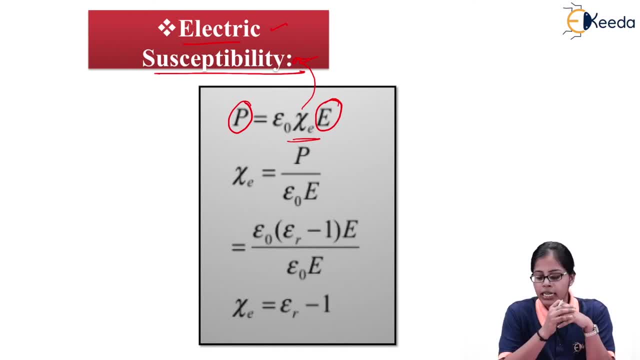 polarized as its subjected to external electric field. that measure is going to be given by the electric susceptibility, which is nothing but denoted by the term or the parameter chi, as it is electric susceptibility. so chi with the suffix a, and the ratio is going to be polarizability divided by absolute. zone naught as this�2 plusоль by xtp, where p-r and the shock state are tan square, so the non square is gonna be positive. there is not this one purpose, so absolutely it's A AND E indicates it's the electric susceptibility. 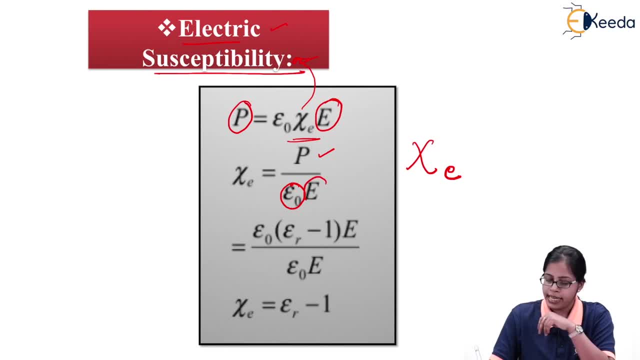 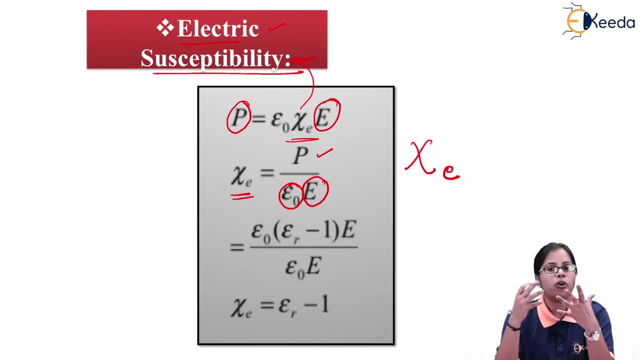 epsilon naught is the permittivity of free space or vacuum. E is the external electric field. So this is the way we get the electrosusceptibility, or the measure of how much the material is getting polarized as it is subjected to the external electric field. So ultimately there 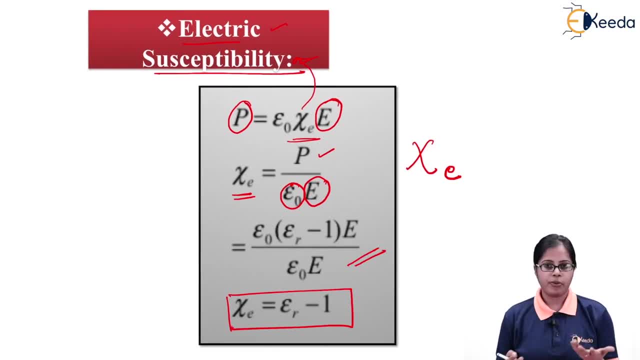 are different forms of writing the same equation. If I want to write chi E, it is one equation. is this Second equation in terms of relative permittivity, that is, in terms of epsilon r? or instead of this I can even write k. k is taken to be the dielectric constant. 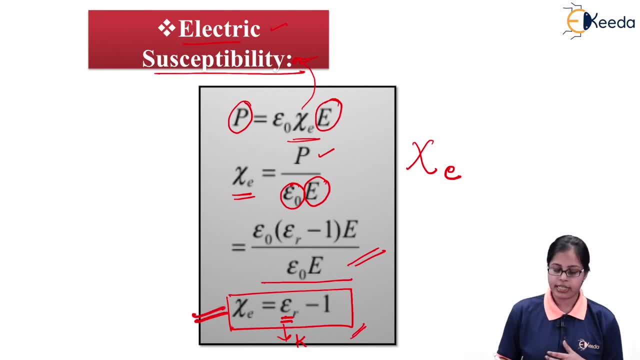 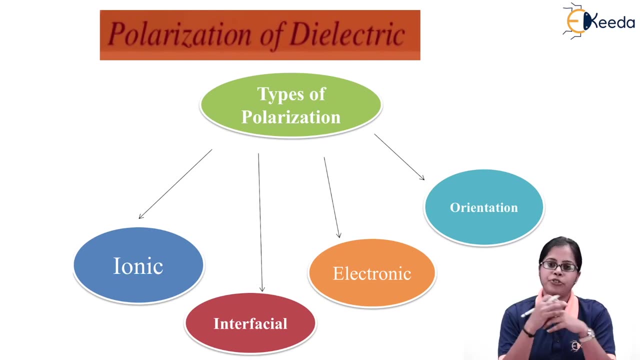 So in terms of k or epsilon r, we can get the equation as chi E. So there are different formulas which are used for finding the chi E terms. Next is, whenever we talk about polarization of dielectric material, there are certain types of polarization. 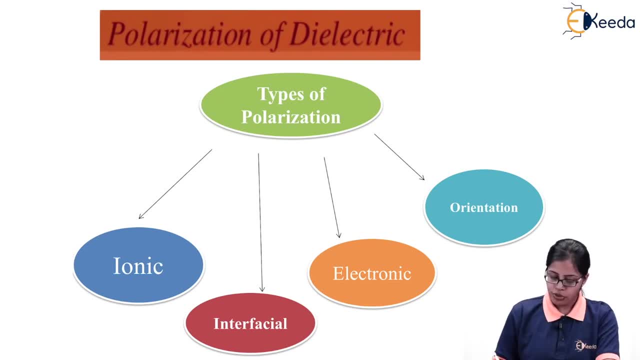 which we commonly use. In this we have shown four types of polarization, That is, one is ionic, second is interfacial, third is electronic and the fourth is dependent on orientation. So this type of polarizations are going to lead to the different types of polarization, or these: 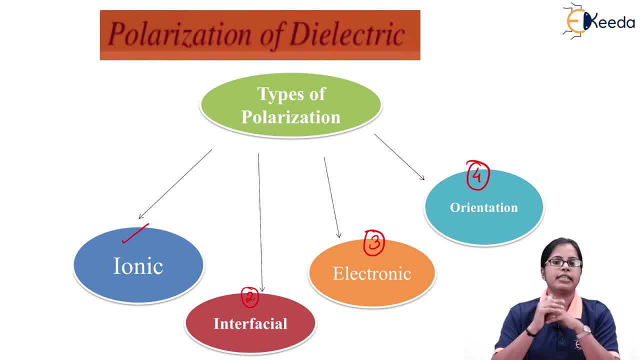 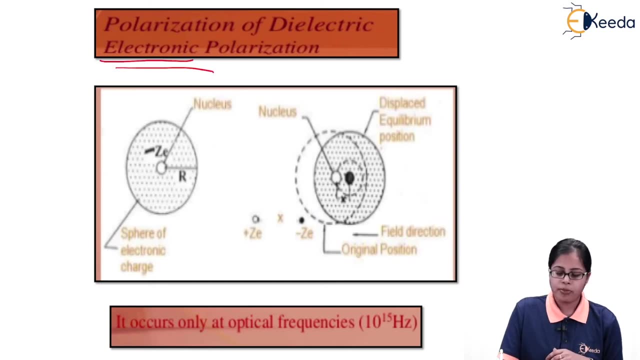 are going to lead to the induced dipole moment inside the dielectric material. So, starting with the first type of polarization, we have the dielectric moment. So we have the dielectric moment, So this type of polarization, that is electronic polarization. Now, what do you mean by? 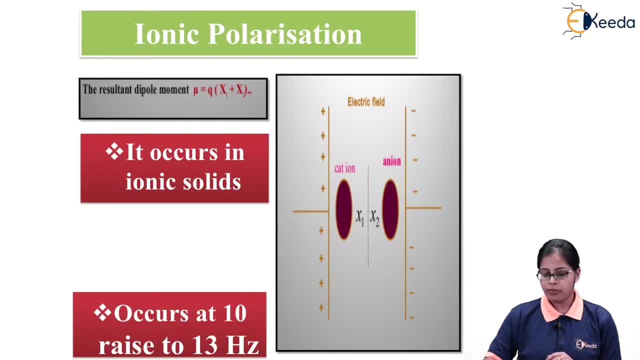 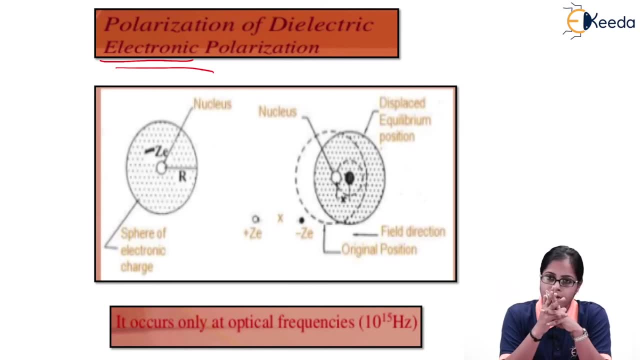 electronic polarization is that whenever we talk about any material, like any material, any dielectric material, they are going to consist of atoms And, as we are aware, atoms consist of a central part called as nucleus and the outer part has orbits which consist of electrons, which 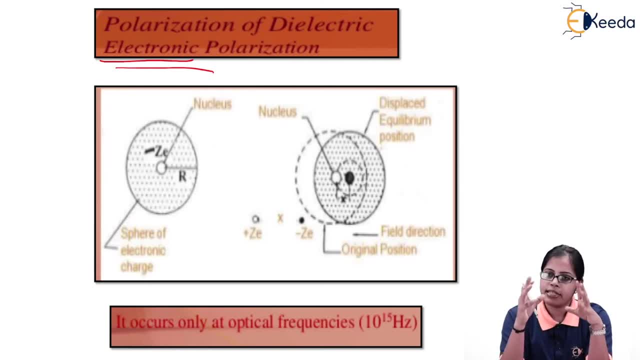 are negatively charged. So this type of polarization is going to lead to the induced dipole moment inside the dielectric material. So whenever we consider the atoms of the dielectric material and during electronic polarization we try to displace the nucleus of the atom from the electronic charges. 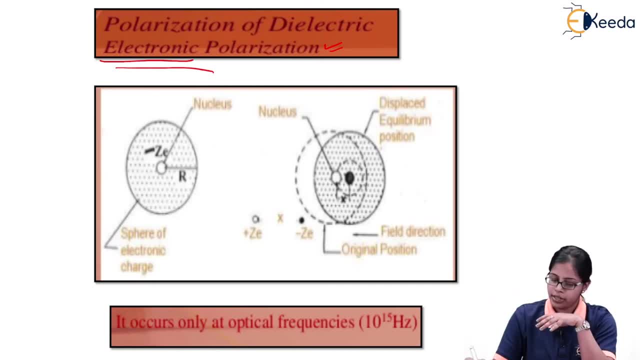 that is electrons. That is, as we are aware, the nucleus are positively charged and the electrons are negatively charged. So whenever we consider the atoms of the dielectric material, we try to displace the nucleus of the atom from the negatively charged electrons. So 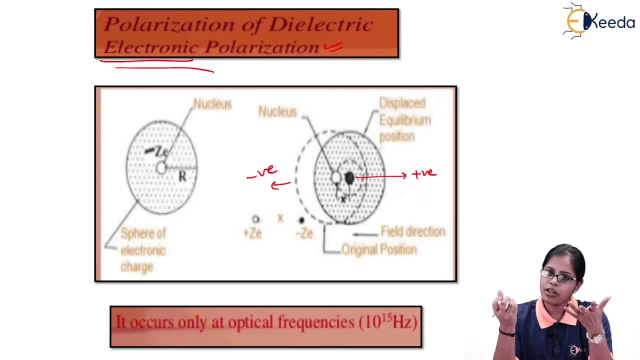 are we trying to separate the positive charge from a negative charge? So if we try to separate the positively charged nucleus from negatively charged electrons, we are displacing them from each other. We are trying to make them away or move them away so that this is going to behave as a positive charge and this is going to behave as negative. 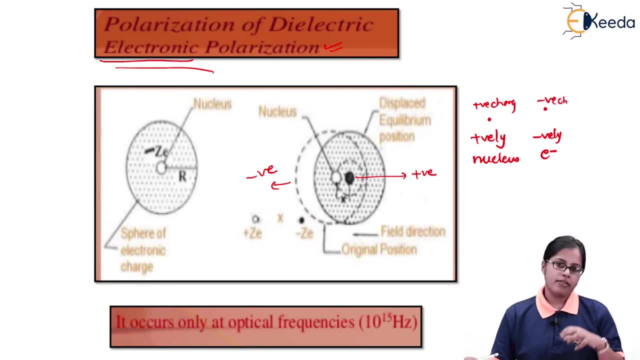 charge. so whenever we try to displace the positively charged nucleus from a negatively charged electron of an atom, we are indirectly displacing or separating two opposite charges from each other which are of obviously equal magnitude. so if i separate the two opposite charges, we are trying to induce electric dipoles in it and the production of a dipole in a dielectric. 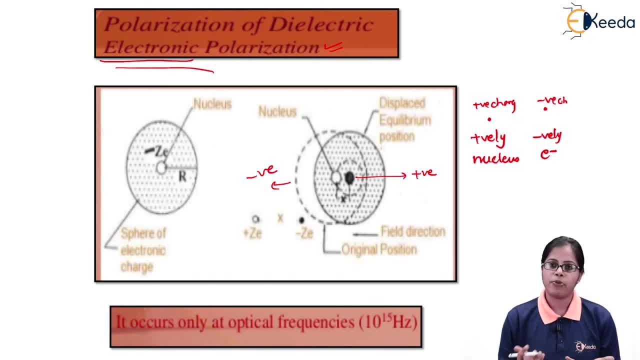 material. that concept of phenomena is called as polarization. so in this electronic polarization we try to separate the nucleus of the atom which is positively charged and we try to separate the nucleus of the atom which is positively charged and we try to the negatively charged electron from each other. and, as you can see, if i'm separating the two, 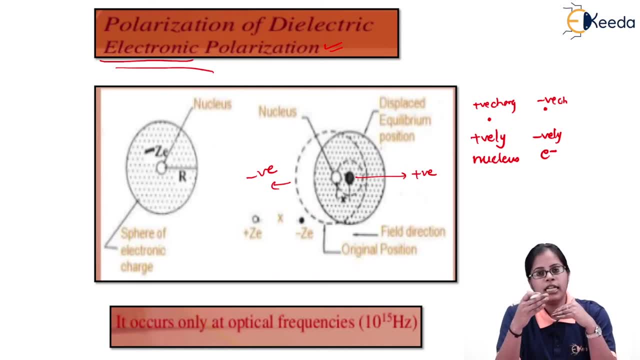 charges or the nucleus from the electron. there is a certain separation between them. that means we can say that if we are trying to displace nucleus from the electron, we are indirectly taking two equal and opposite charges separated by certain distance. we are trying to induce dipole in the dielectric material, so we are trying to displace the two opposite charges. 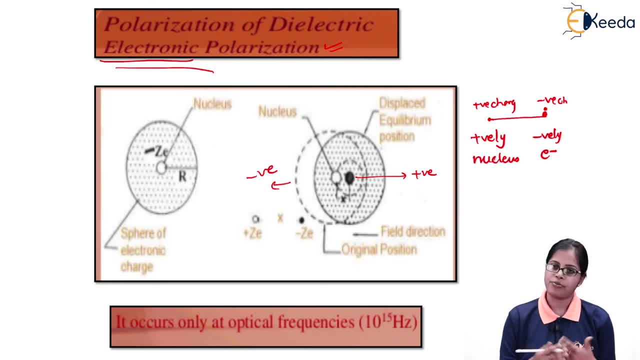 from each other by a certain finite distance. we are trying to induce dipoles in the dielectric material. this type of polarization is called as electronic polarization. that is, separation of positively charged nucleus from the negatively charged electrons, leading to the induced dipole moment in the dielectric material. this type of polarization is called as electronic polarization. 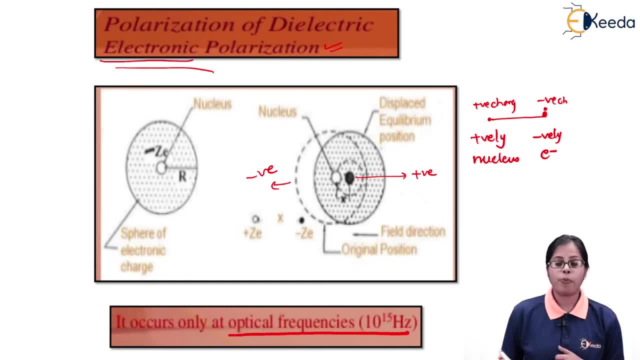 and this polarization occurs at an optical frequency of 10 raised to 15 hertz. you have to keep in mind that this polarization is not available at all the frequencies. it is only applicable at 10 raised to 15 hertz. firstly. secondly, this type: 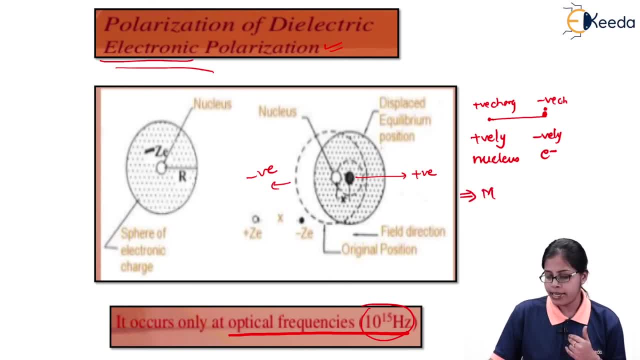 of polarization is preferable for monoatomic gases. so whenever we consider monoatomic gases and that the electronic polarization undergo firstly and secondly, thirdly, we can say that this type of polarization is completely independent of temperature. so this type of polarization is completely independent of temperature. so we have to remember the basic parameters which are used for the electronic polarization. 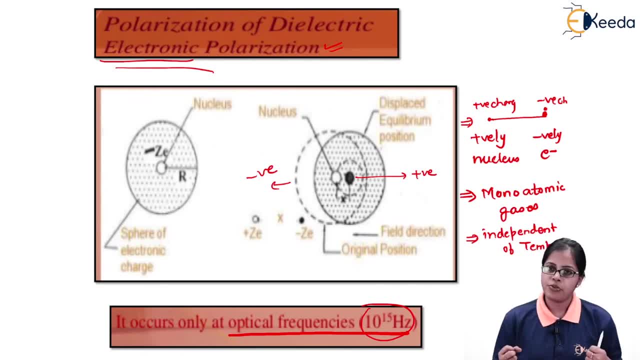 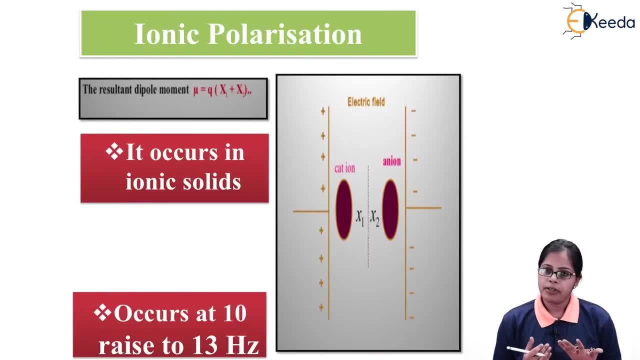 so simple separation between the positively charged nucleus from the negatively charged electron is going to lead to electronic polarization. next is when we talk about ionic polarization. in this case, first of all, this type of polarization occurs in ionic solids. that means, if i have a positively charged ions, 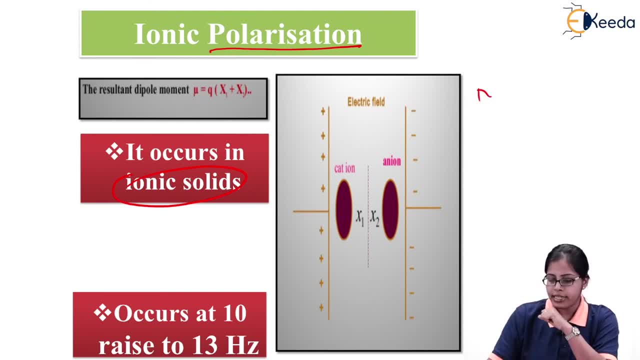 and negatively charged ions. for example, if i consider a compound that is NaCl, which is having or we can say, which is made up of two ions, that is, sodium, positive ion, and chlorine negative ion, that is, cations and negative ions, in that case, when i consider these two ions, 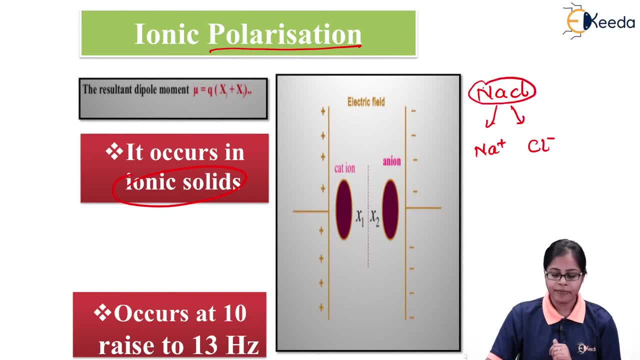 and if they are together in a form of NaCl, and if we subject this NaCl material to an external electric field, what is this external electric field is going to do? is it is going to separate the NaCl into Na plus, that is positive ion, and Cl minus, that is negative ion. 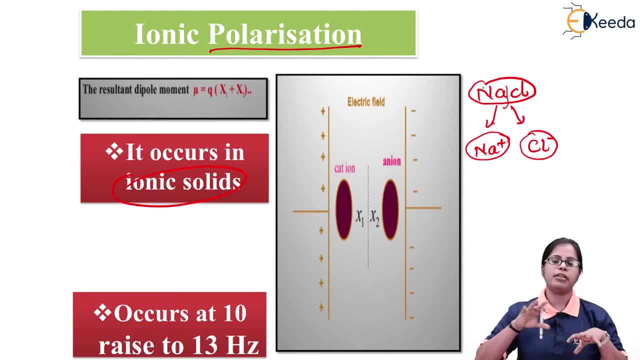 so if we are separating positive ion from a negative ion and if they are getting separated from each other from a certain distance, that type of polarization is called as ionic polarization. so we can say that this occurrence of ionic polarization occurs only in ionic solid. first, 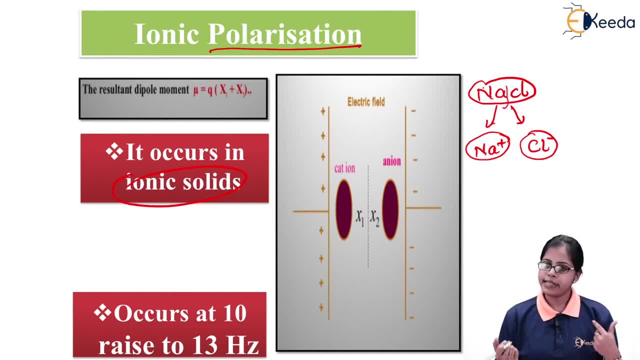 of all. secondly, how does it going to occur is whenever we try to separate positive ion of the solid from the negative ion of the solid, so we are separating positive ions and the negative ions. this leads to the formation of electric dipole, and this type of polarization is ionic polarization. 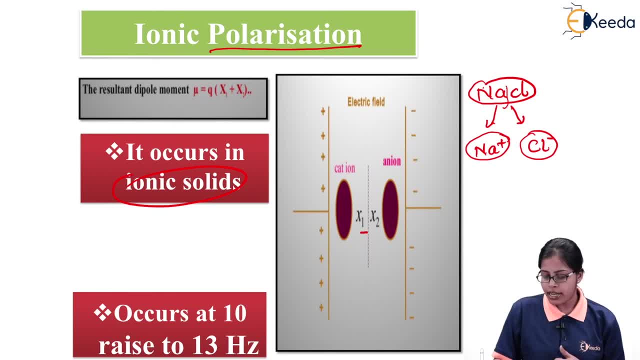 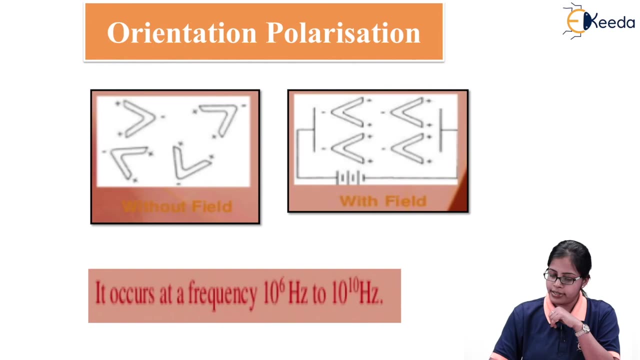 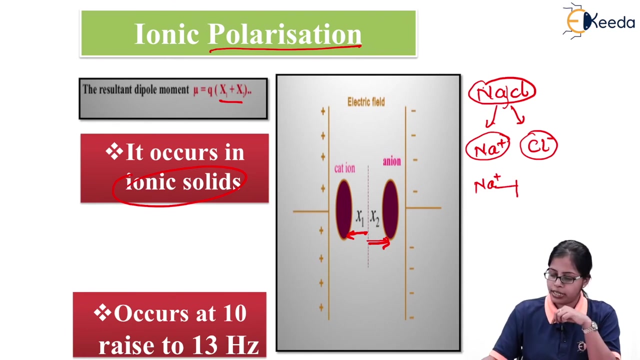 as you can see, the displacement of cation is x1 and displacement of anion is x2. so if you take, the overall displacement is going to be x1 plus x2. this is the total distance between the two ions. so cations, that is, Na plus, has been displaced from a certain equilibrium position, that is. 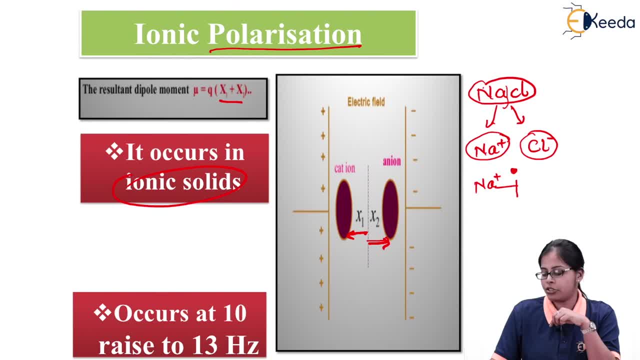 from. suppose, if i consider this has an equilibrium position. from this equilibrium position, Na plus has displaced x1 distance and from this again equilibrium position, Cl minus has displaced by x2 distance. so this is your positive ion and this is indicating the negative ion. they both are, overall, separated by the total distance of. 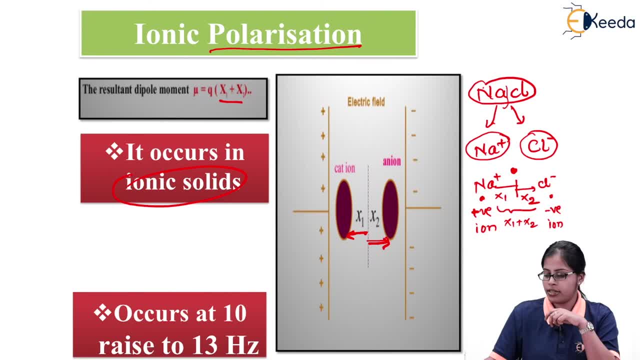 x1 plus x2, that is the total distance of x. and this separation of two equal and opposite ions from each other with a certain finite distance between them is going to lead to the formation of electric dipole. and this Na plus has been displaced to the final distance of self-correction of the 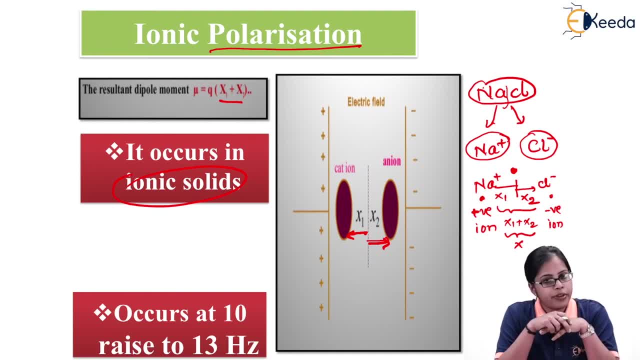 And this whole process is going to be called as ionic polarization. So if you look at the whole ionic solid, it is your NaCl material which is getting classified into two types, that is, Na plus and Cl minus. The displacements, respectively, are X1 and X2.. 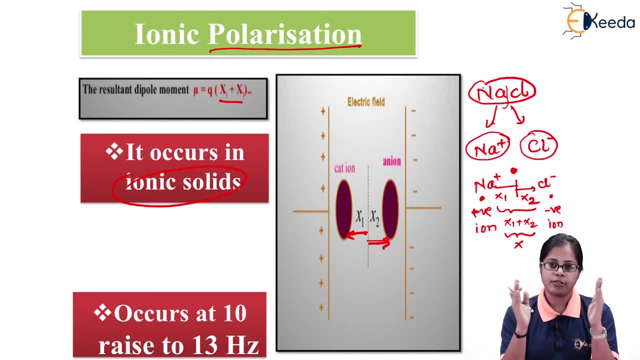 So the finite distance between the two ions that is positive and negative is your X. So if I take this total distance when the two ions is X1 plus X2 times the charge, it will give me the resultant induced dipole moment. 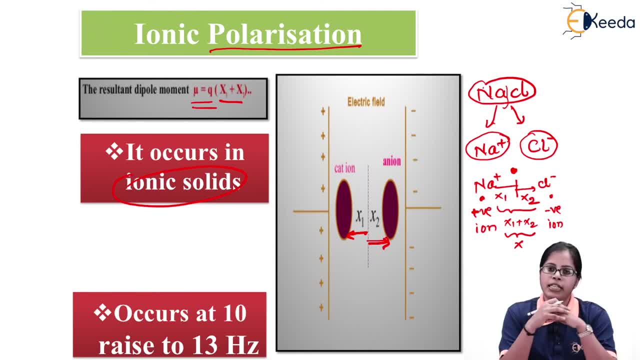 Because, if you remember, the dipole moment is nothing but the product of charge into distance. The charge is going to be Q and the total distance between the ions is X1 plus X2.. So this is the way we are trying to displace the ions from their equilibrium position. 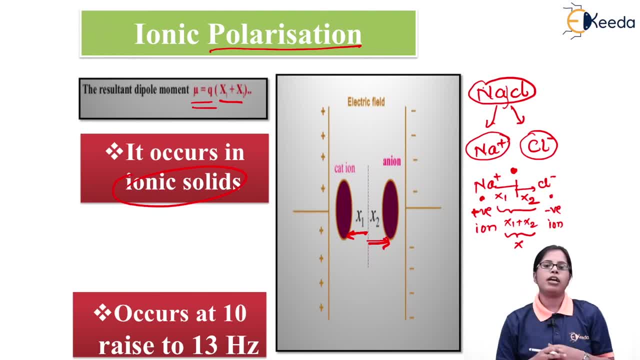 And these ions are separated. They are separated by finite distance leading to the ionic polarization, And this polarization occurs at frequency of 10 raised to 13 hertz, firstly. Secondly, ionic polarization occurs slower than electronic polarization And, secondly, it is independent of temperature. 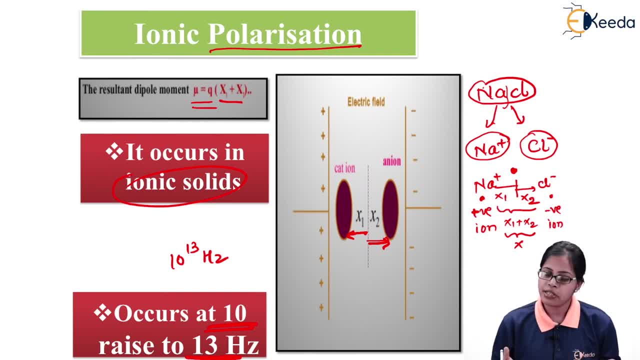 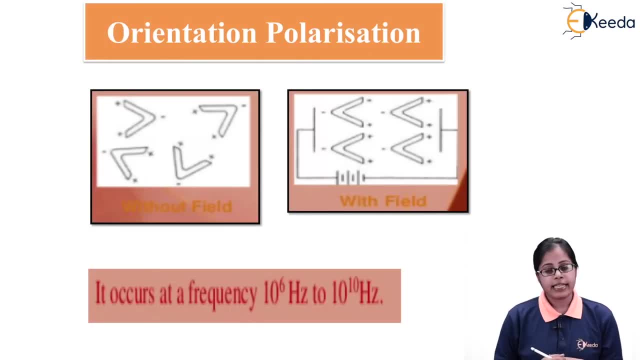 So if it is asked which polarization is going to be faster, the electronic polarization is much more faster Than your ionic polarization. Next is third type of polarization, which is called as orientation polarization. Now, specifically, this orientation polarization occurs only in polar dielectric material. 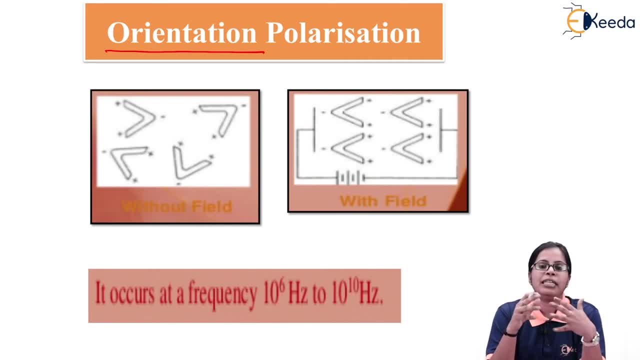 Means the dielectric material, which consists of only polar molecules. in that type of dielectric material the orientation polarization is going to occur. So please keep in mind that orientation polarization basically occurs in polar molecules of the dielectric material. firstly, 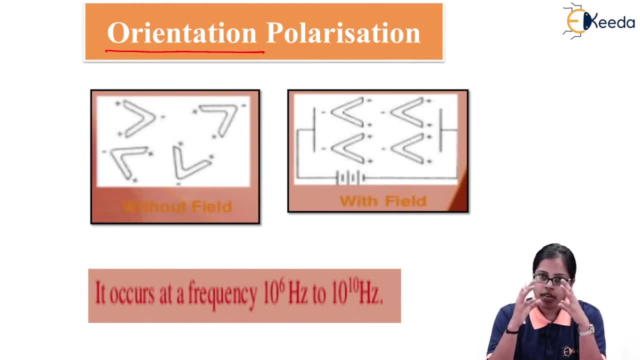 Secondly, in this case, whenever I consider a polar molecule, it has a permanent electric dipole present in it. As we have already discussed this in the previous concepts, that polar molecule always has the presence of permanent electric dipole, With the absence of external field or without the external electric field. the orientation of the dipoles are random. 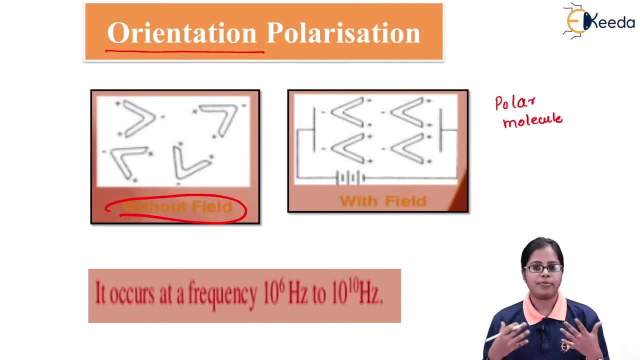 So if the orientation of dipoles in the absence of external electric field is completely random, even if the dipoles are present, Then they are going to cancel out each other, giving me no dipole moment. That is, the dipole moment is going to be zero. 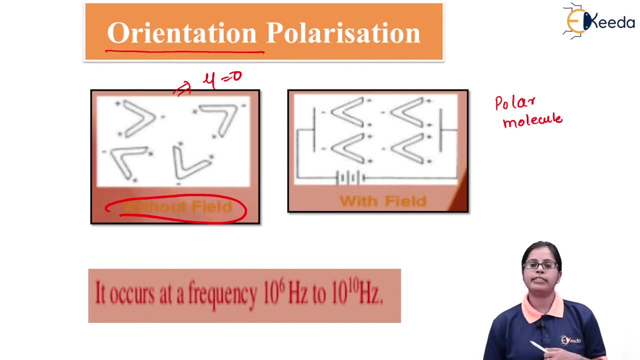 Why? Because we have considered a polar molecule which has the presence of permanent electric dipole. But even with the presence of permanent electric dipole, as we have absence of external electric field, the orientation of the dipoles are randomly oriented. 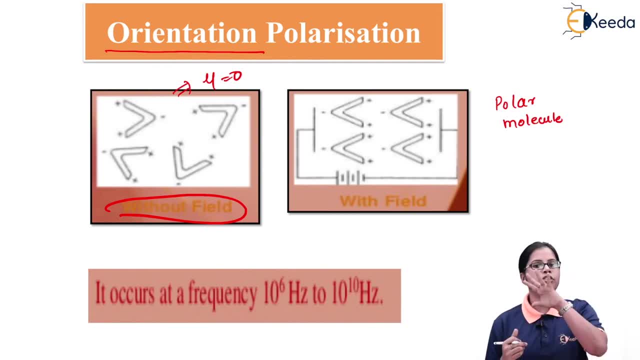 As they are randomly oriented, the charges are going to cancel out each other, or the dipoles are canceling out each other, giving me the net dipole moment to be zero. But if I subject that same polar molecule having the permanent electric dipole in it, 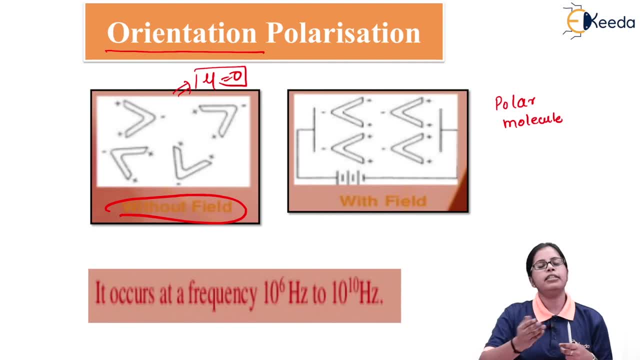 if I subject it to an external electric field. in that case all the dipoles which were previously randomly oriented, they all get oriented in a direction of external electric field. Now, if the alignment of dipoles occurs in the direction of external electric field, 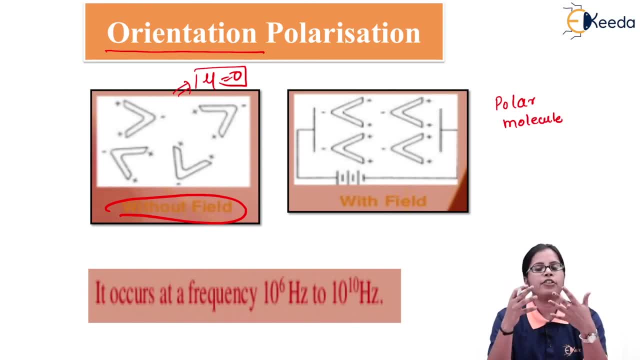 this will give rise to induced electric field inside the material, leading to the polarization of the material. So in this case, if the dipoles are getting oriented in the direction of external electric field, so the induced or the net induced dipole moment is not going to be zero. 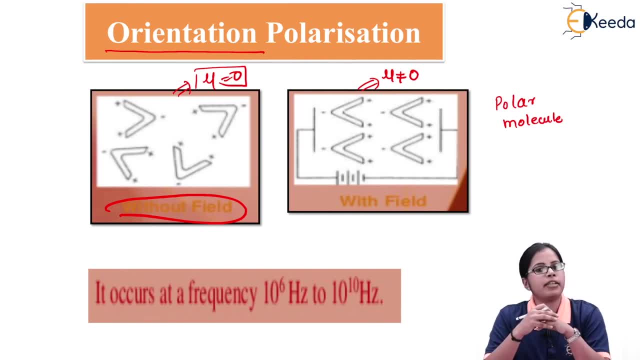 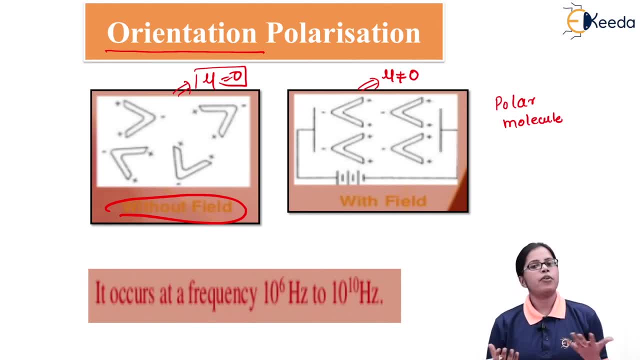 If I don't get any induced dipole, moment that material is unpolarized. If I don't get any induced dipole, moment that material is unpolarized. So if we look at orientation, polarization in this case, it firstly occurs only polar. 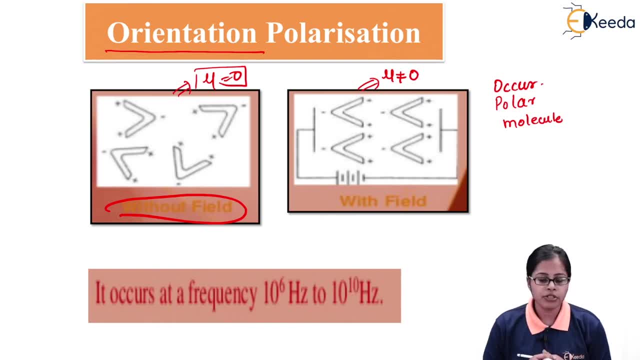 molecule as they have presence of permanent dipoles. But in the absence of external electric field, the permanent dipoles are randomly orientated, so canceling out each other. and as soon as we subject it to external electric field, the dipoles get aligned in the direction of external electric field, leading to the dipole. 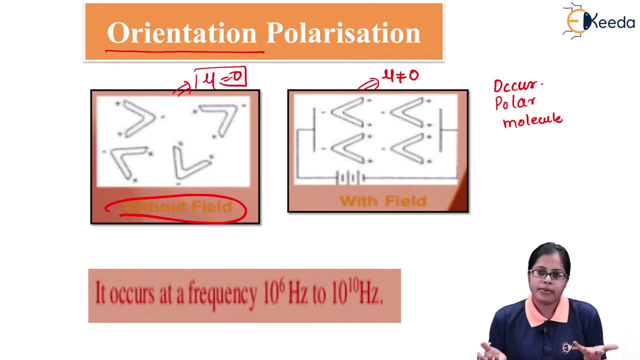 moment. So this is called net dipole moment. and if I get a net dipole moment we can say the material is getting polarized. So this type of polarization is called as orientation polarization. Secondly, this polarization occurs in the frequency range of 10 raised to 6 to 10 raised. 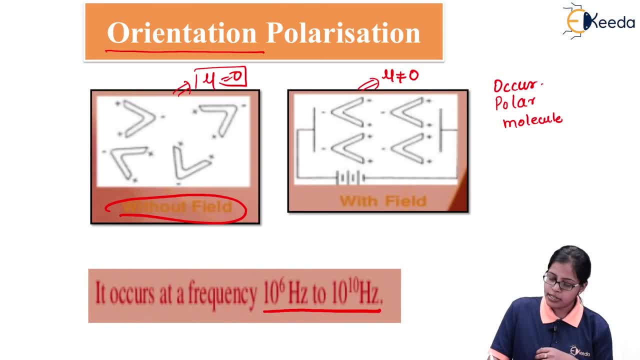 to 10 hertz. Thirdly, this orientation polarization is dependent on temperature. As I said, the previous two polarizations were independent of temperature, is that is, the electronic and the ionic one. but the orientation polarization is entirely dependent on temperature and when we talk about the activity rate, that is, it is going to be slower as compared. 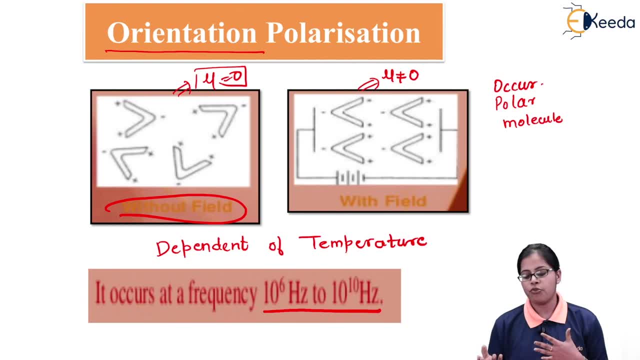 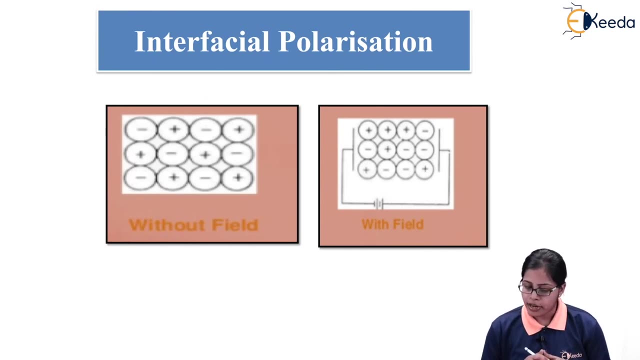 to the ionic polarization. so if we want to talk about the time consumed, it is going to make take more time as compared to the ionic polarization. the last type of polarization is interfacial polarization. now, as you can see the charges over here, that is, negative and positive charges up. 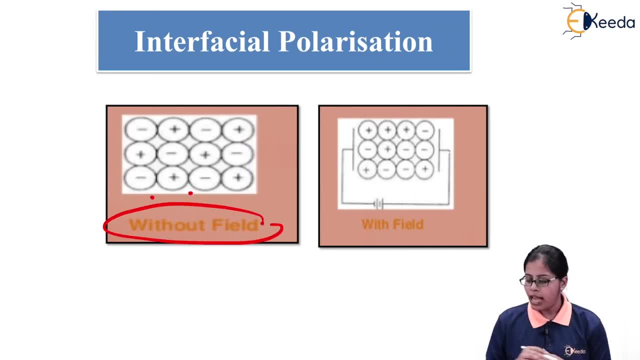 randomly oriented without the field, and with the field they get a proper alignment. now, when does this interfacial polarization occur? or what do you mean by interfacial polarization? the? this is nothing but the accumulation of charges at the interface of the material. when we say: 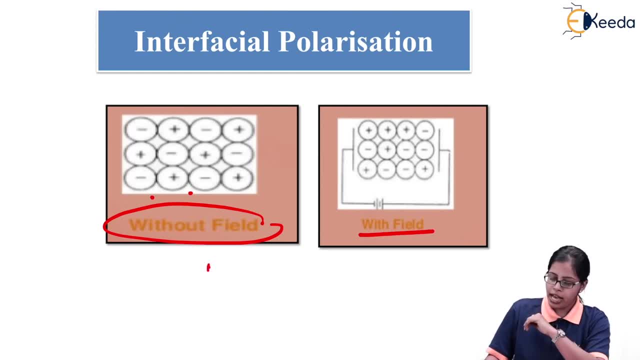 interface of the dielectric means what like if i have a slab which is consisting of compound dielectric. when i say compound dielectric means more than one dielectric. so i have a slab which is made up of compound dielectric, so there will be a boundary which separates the two dielectric. 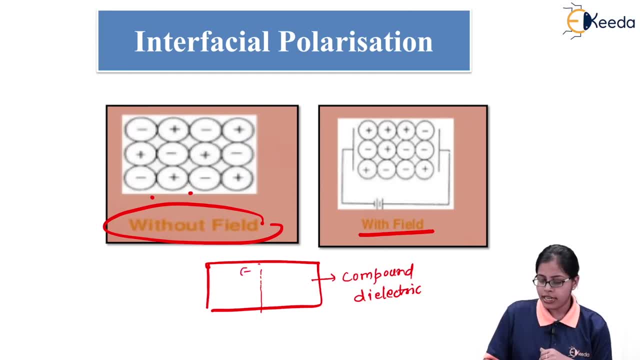 from each other. in that case the charges will be accumulated along the interface or at the interface of the dielectric material. so if there is an accumulation of charges at the interface of the material or the separation between the two materials, it is going to be leading to the polarization called as interfacial polarization, but without 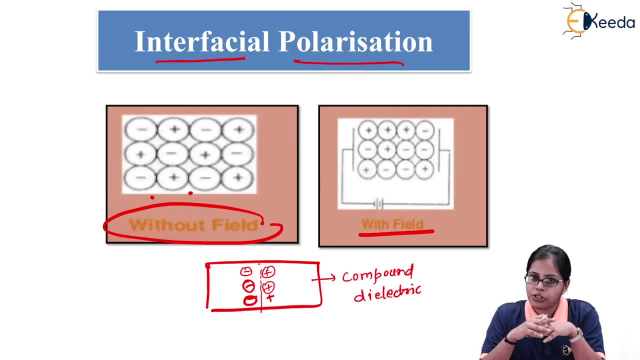 the external electric field there will be no accumulation of the charges. but as soon as we subject that material or the dielectric material to an external electric field, it leads to the accumulation of charges at the interface of the compound dielectric. so if there is an accumulation of charges at the interface or the boundary between the two materials, 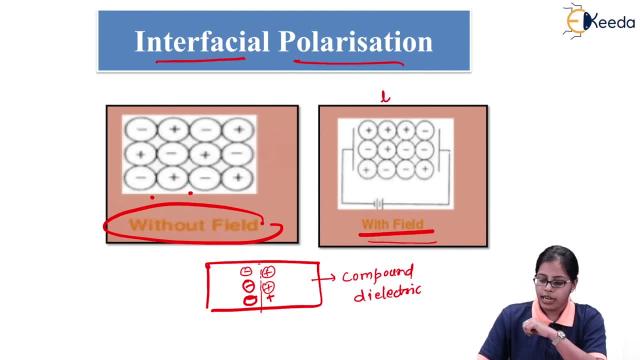 this leads to the formation of induced dipole moment. So if I get an induced dipole moment, that means the material is getting polarized. that type of polarization is considered to be interfacial polarization. So this interfacial polarization mostly occurs in compound dielectric, that is, having more than one dielectric, or you can consider basically the dielectrics having the interface between them, boundary between them. 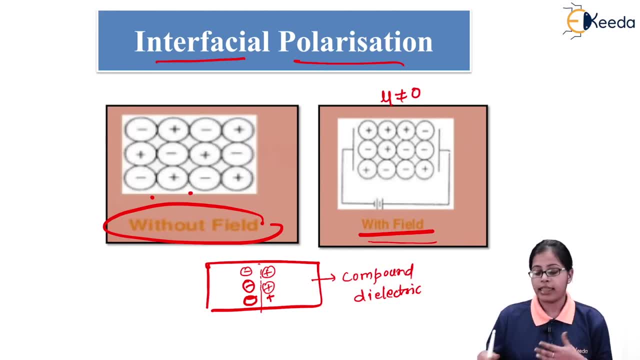 And at the boundaries there is an accumulation of charges, and that accumulation of charges will lead to the net dipole moment to be non-zero. And if I get the net dipole moment to be non-zero, that means the material is getting polarized. 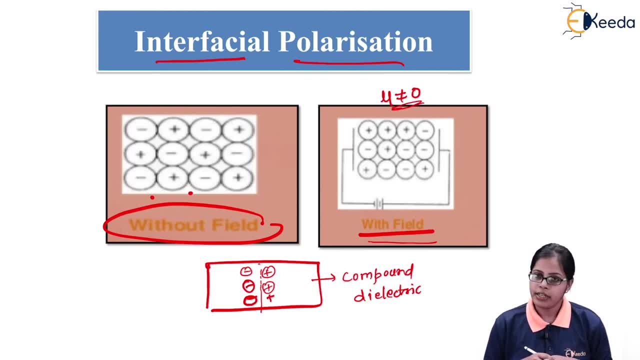 So this is the last type of polarization which can occur. So overall, when we talk about the dielectric undergoing polarization, we can have four types, that is, electronic, ionic, Third orientation, And the fourth is interfacial polarization. 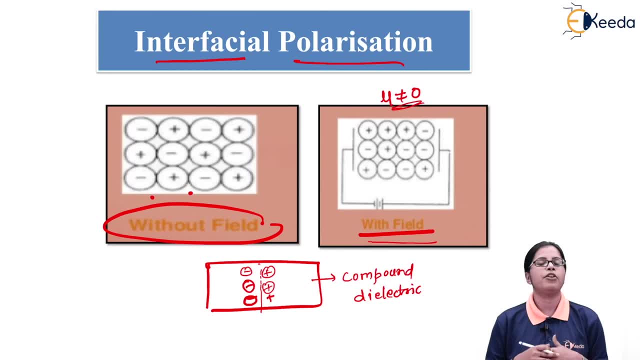 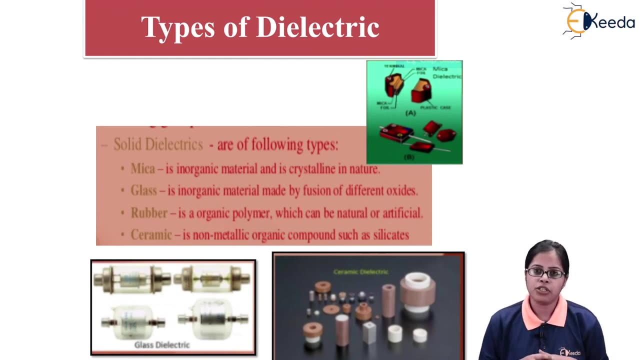 So this is all about the polarization concept, or the phenomenon of inducing dipole moment in a dielectric material with the help of extra electric field is about. Next is when we talk about this dielectric materials and the phenomena that is polarization, obviously we need to consider the types of dielectric material which are present in nature. 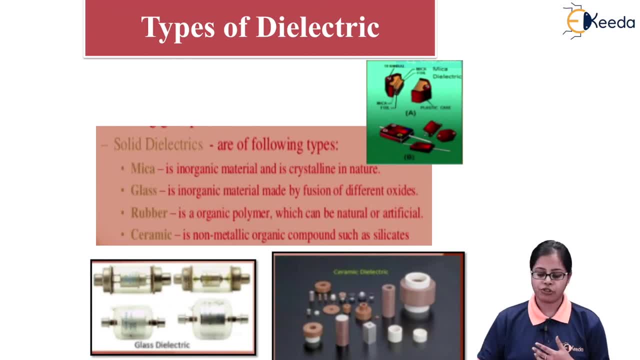 We have many types of dielectric, Like in this case. I have shown solid dielectric Which are nothing but mica, glass, rubber ceramics. These are considered to be the solid dielectrics which are present in crystalline form. 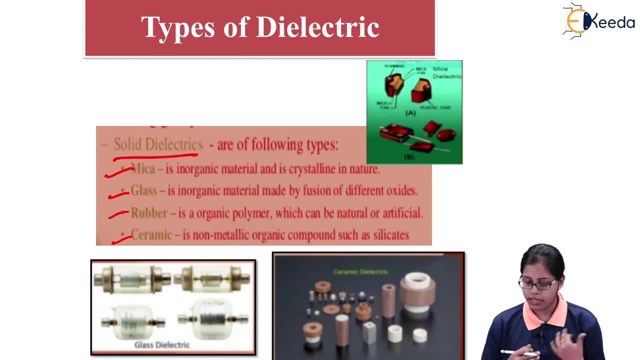 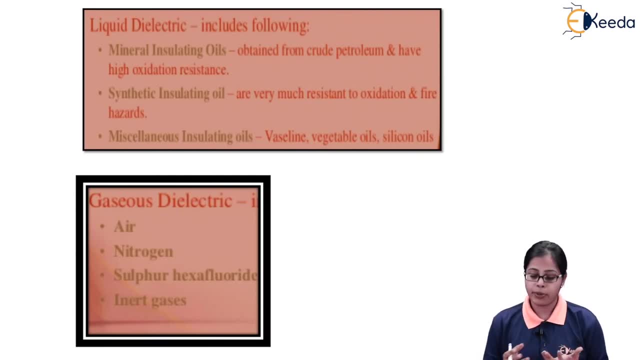 They can be inorganic, They can be organic polymers, They can be non-metallic, So, accordingly, these are the solid dielectrics. In a similar manner, there is a presence of liquid dielectrics in a form of mineral insulating oils. 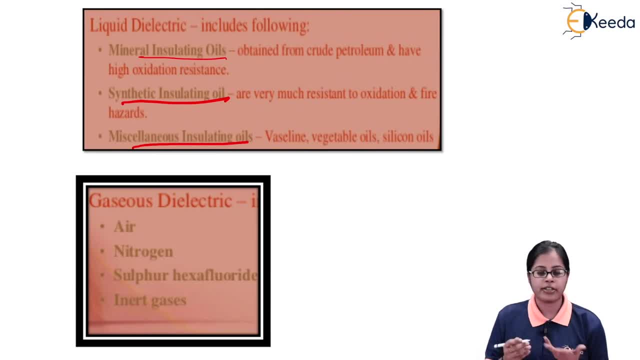 We can even have synthetic insulating oils and the miscellaneous insulators, That is, vaseline and oil. They all are considered to be the dielectric material, but liquid dielectrics. And lastly, when you talk about gaseous dielectric, the most basic dielectric in terms of gaseous is taken to be air. 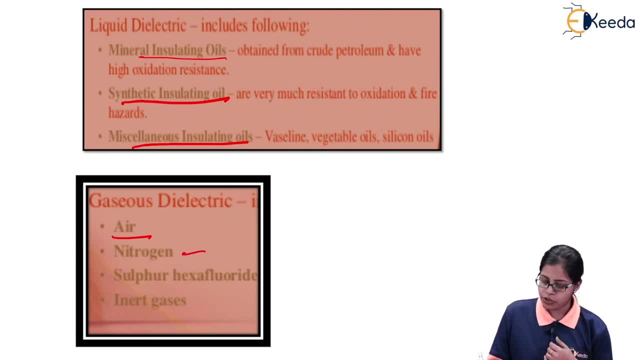 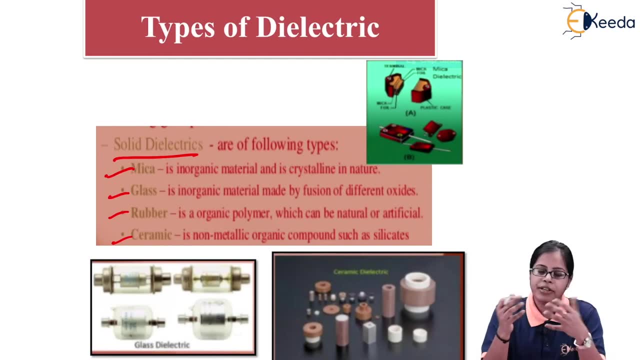 And obviously there are many more gaseous dielectrics, That is nitrogen, sulfur, hexafluoride, inert gases. So we can say that the dielectrics are present in all the three forms. That is solid dielectric. 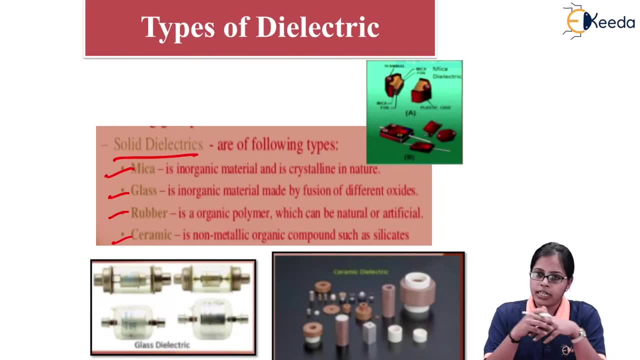 Liquid dielectric and the gaseous, But most certainly the dielectrics which we see in the nature, is your air, because air is also an insulating material. Or you can say, air also behaves as a dielectric, which is a gaseous type of dielectric. 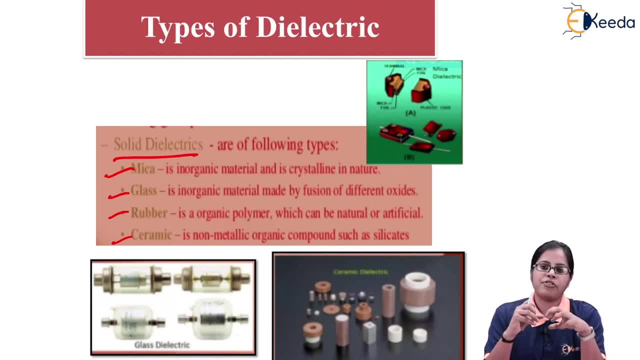 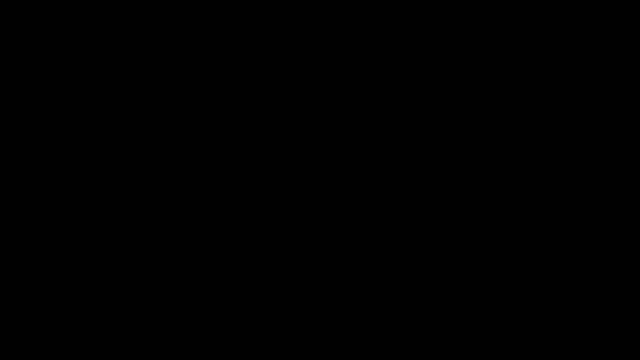 So with this video you are clear about the concept of dielectric and the phenomena called as polarization. So that's all for this video. Thank you so much. Thank you. 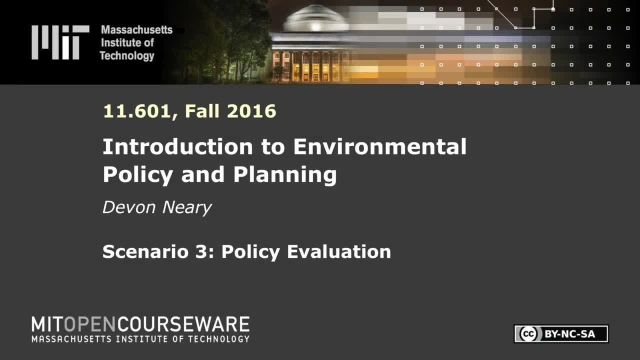 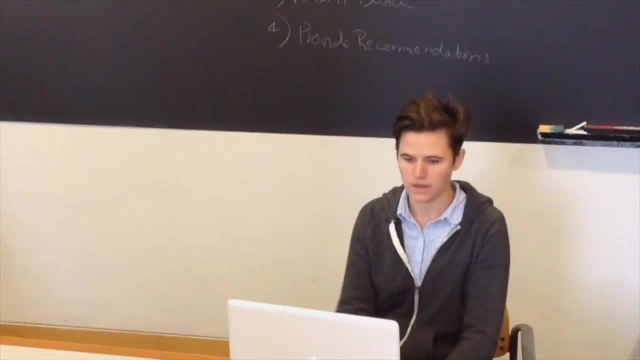 Dear Secretary of the Interior, thank you for inviting me to weigh in on this very important counter-study to an indefensible claim by the Heritage Society. As you know, this conservative organization is pushing for free enterprise and limited government, So they're merely. 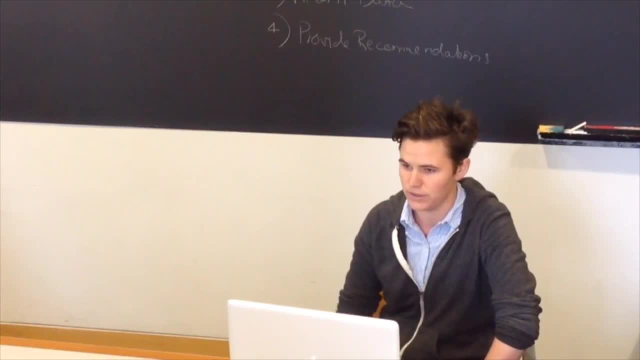 trying to deregulate, to support free enterprise and to help their allies, including industries, to save some money. As you know, in 1970, the EPA was formed to control the extreme pollution of water and air in this country. These conditions were causing fish kills.